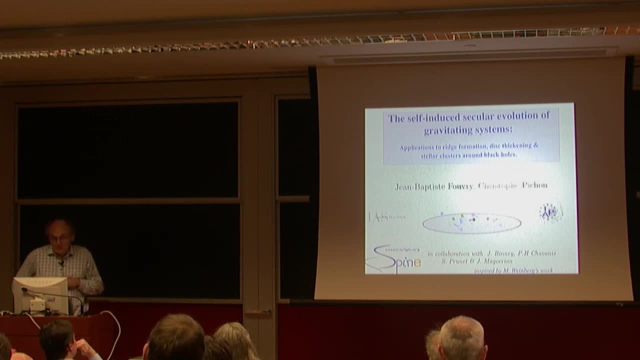 Balisculinar equation and I aim to show in this presentation that this equation provides a stochastic framework which can complement or rival possibly a classical n-body framework. It opens in particular the possibility of following semi-analytically the complex dynamics. 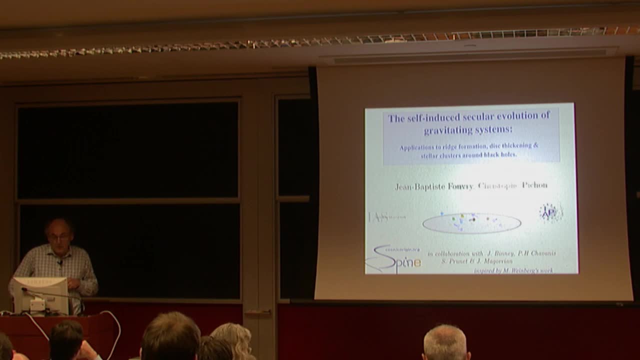 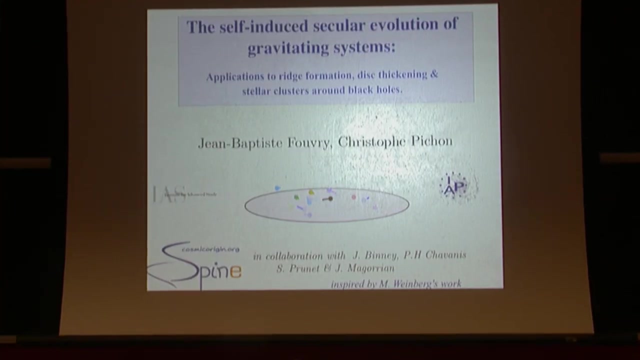 of self-gravitating system over a long time, a Hubble time in cosmology, and this is unprecedented for a cold or tepid system. So I will go from the general to the particular and from galactic dynamics in the broad sense to the stellar dynamics of the nuclear clusters, which is 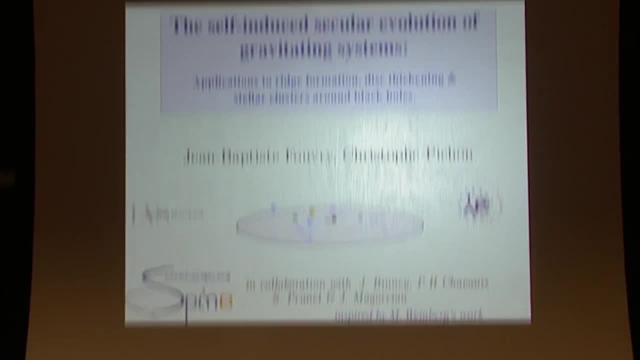 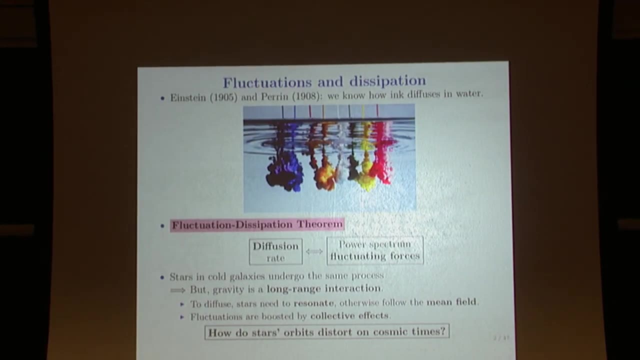 the focus of this workshop and hope to convince you that these so-called kinetic theories can help you understand the dynamics of the nuclear clusters. I hope to convince you that these so-called kinetic theories can help you understand the dynamics of the nuclear clusters. I hope we'll be able to address key questions in galactic and nuclear dynamics. 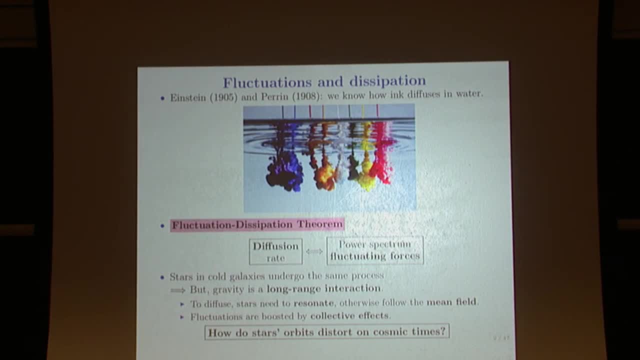 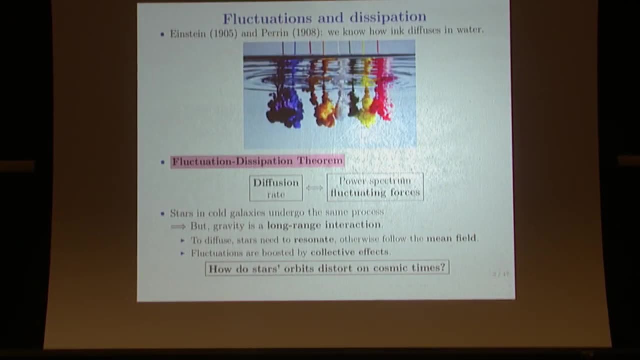 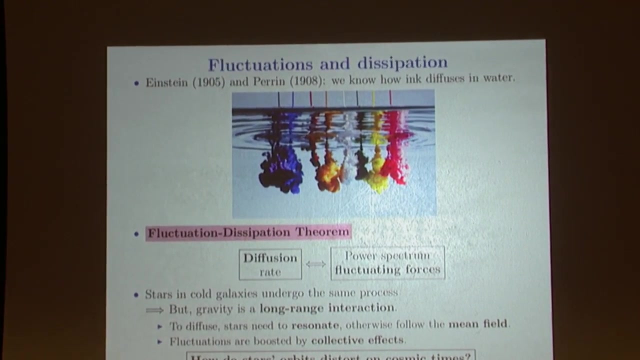 So as following the previous question. the origin of this equation arises from the transposition of Brownian motion in the context of self- gravitating systems. Since the work of Einstein and Ther л, we understand how ink diffuses in water and the process reflects a very general principle in physics known as the fluctuation-dissipation. 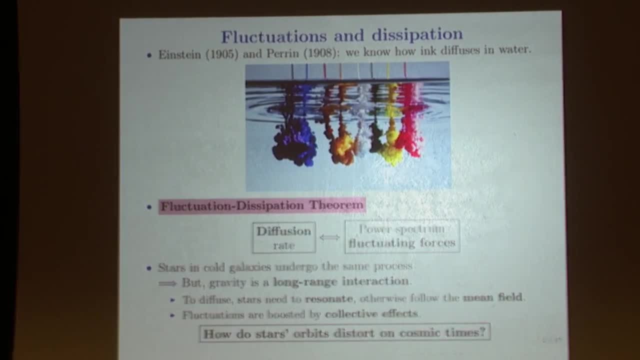 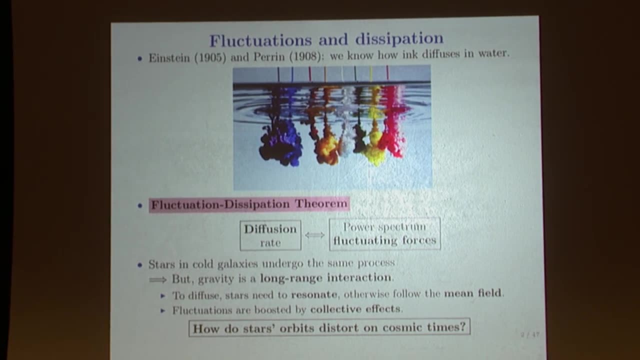 theorem which basically relates the rate of diffusion of something to the correlation- Correlation of the fluctuating force responsible for the diffusion process. So the key idea is that typically hydrodynamical and radiative processes lock, by symmetry, self-gravitating systems into a state of low entropy. 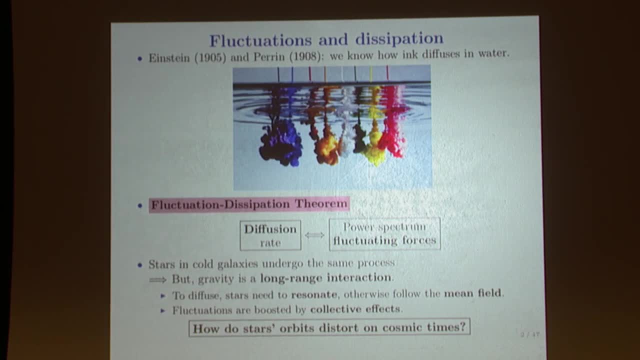 where stars follow unlikely quasi-circular trajectories imposed by the mean field, And I will show that through resonance these stars can start to feel each other and eventually distort their own orbits. This corresponds to diffusion in orbital space. This is what we call secular evolution. 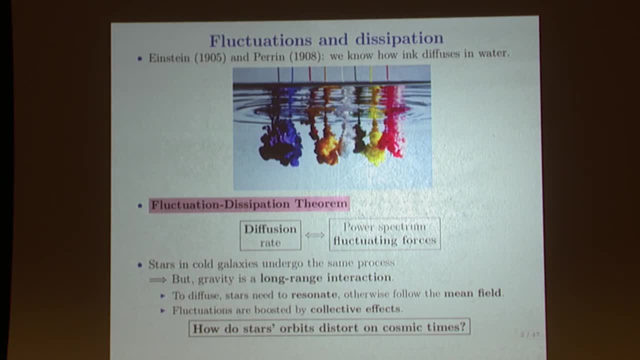 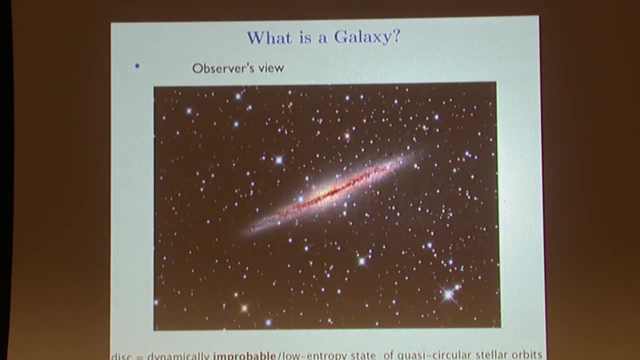 the slow process by which a self-gravitating system evolves towards more likely states through fluctuations of the potential. So, as promised, I will start with galaxies in general, so as to later draw your attention to the specifics of galactic centers, since, in some sense, the general problem is simpler than the problem of the galactic center. 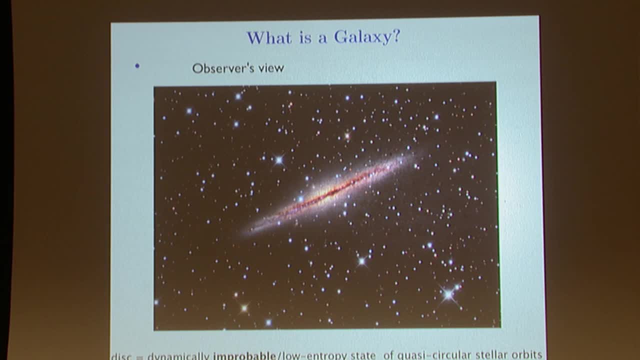 So we want to explain how this object will evolve on conservatively. It will evolve on cosmological timescales through self-interaction of its component. So, technically, our purpose is to explain things like radial migration and blurring and shurning in the context of the Gaia mission or galactic archaeology. 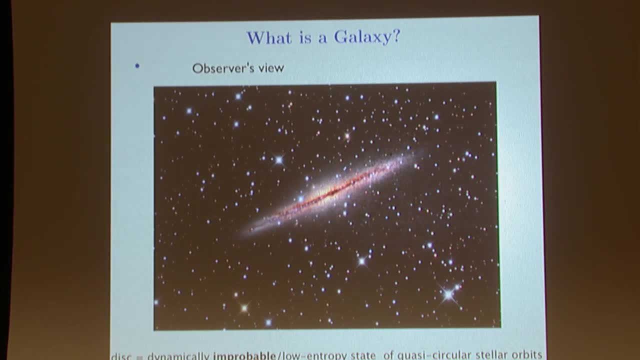 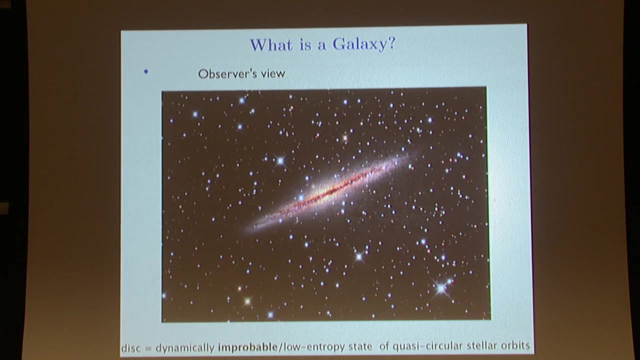 or something people also call near-field cosmology. So a key property of thin galactic disks such as NGC 891 is that its formation process has set it up into a dynamically improbable low entropy state of quasi-circular stellar orbits, And this is the result of shocks and radiation coming from the fact. 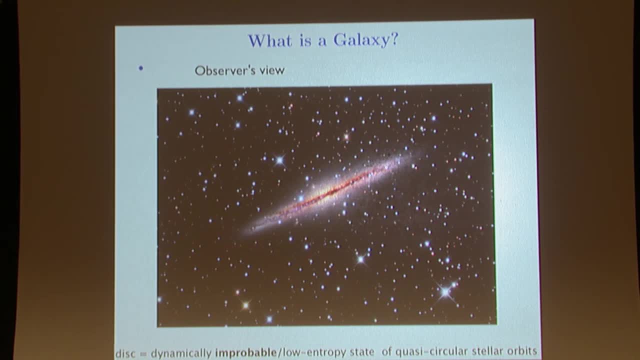 that the stars were built from the past gaseous component. So, given a Hubble time, it can and will therefore easily adjust its structure via resonant encounters so as to explore more likely configuration. So the purpose of this talk is: can we explain this from first principle? 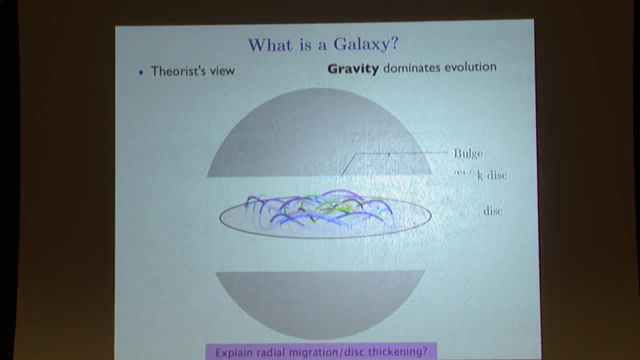 So, for the sake of this work, I will consider the following idealized framework of a thin and thick disk. This is a disk embedded in a dark halo, and I will assume that gravity dominates the collisionless dynamical evolution of the stellar fluid. While this level of description is crude, the motion of the stars within such a system are complex. 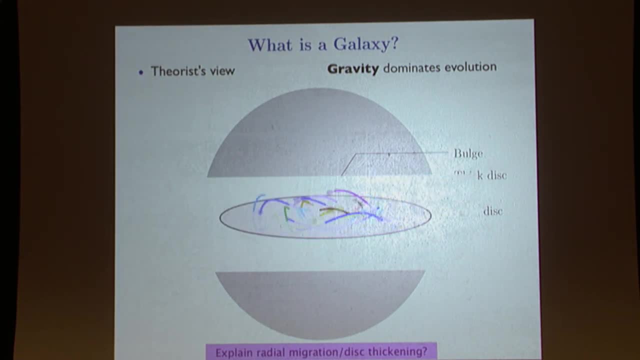 and this is something that we will need to address in order to predict its long-term behavior. So how can we predict the self-interaction of these stars on a very long timescale? And the key here is to identify a recurrence which will allow the perturbation to grow up. 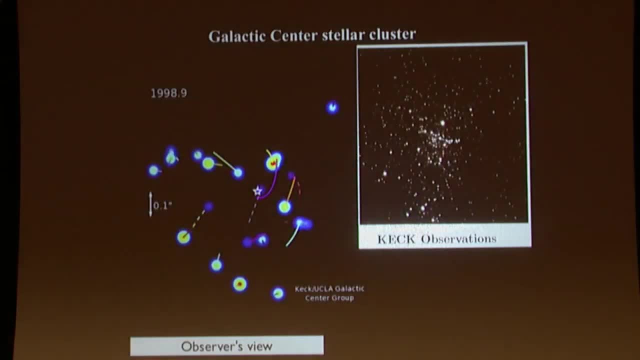 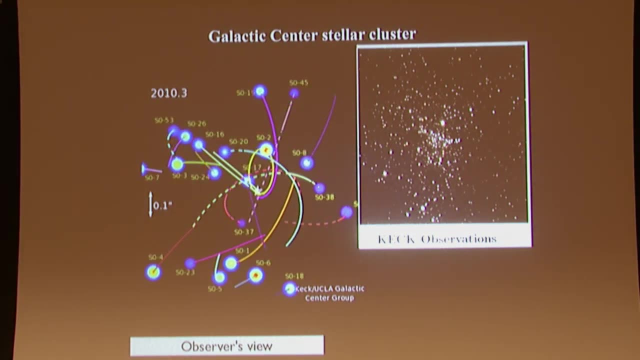 and that's through the recurrence. Okay, So this is an example of what we can do to predict the self-interaction of these stars within a very long time scale. So we will also obviously talk about the galactic center, and here the motion of the S-cluster is Keplerian to first order, but we may wonder what the effect. 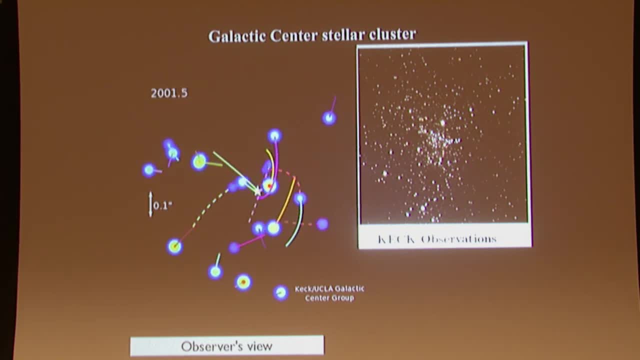 of relativistic corrections from the massive central object will do on long timescales and what the mass of the cluster itself will do on the evolution of this system. This is all the more important on galactic scales, on nuclear scales. so the guy element can can't actually do much in the pulse measurement information. 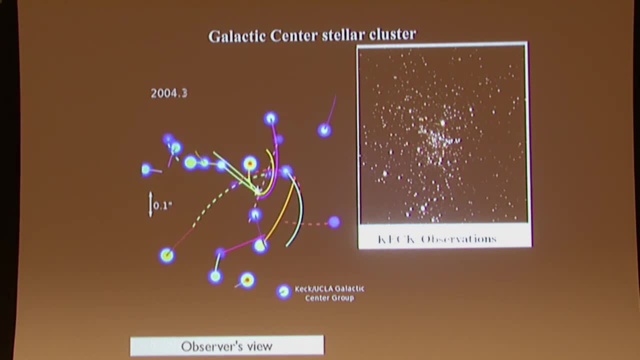 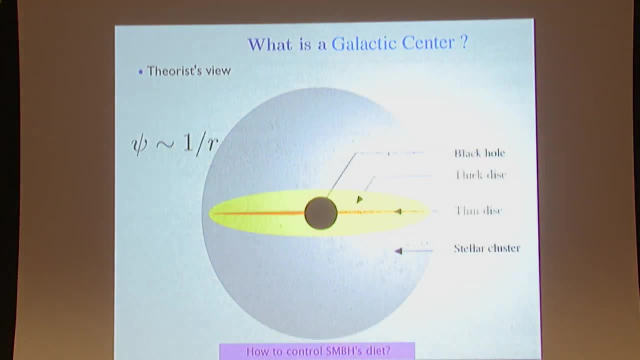 Indeed, there is evidence that it cooking in the腱 rate, bothQuery and potential, is special. so the challenge in this context is to explain why a black hole doesn't hit too much of its environment, not too little. So we have a fine-tuning problem of explaining what happens to the stars in its vicinity. 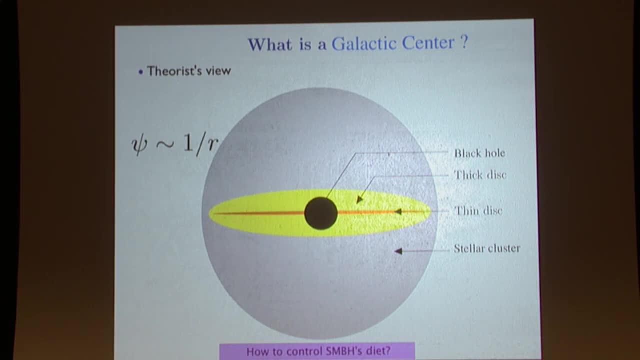 So, again, the abstraction will be the same. Well, I'm going to, in fact, to focus on a flattened stellar cluster orbiting the black hole, is that the potential is essentially Keplerian, and this involves an extra complication because it induces degenerate frequencies. so we'll have to. 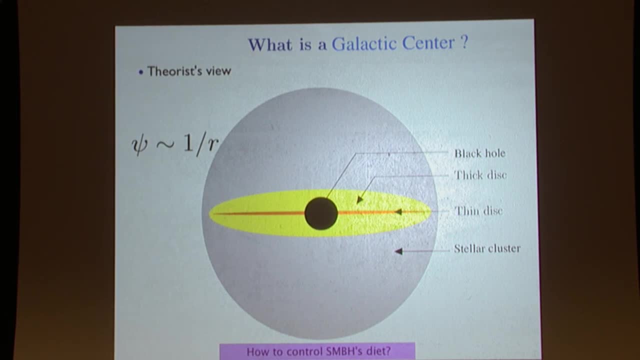 circumvent this difficulty, which is what is specific to a secular evolution in the galactic center. so if I have time, I'll say a few things about the situation where the black hole might be spinning or the stellar cluster might be non-spherical in the vicinity of the black hole, which induces different 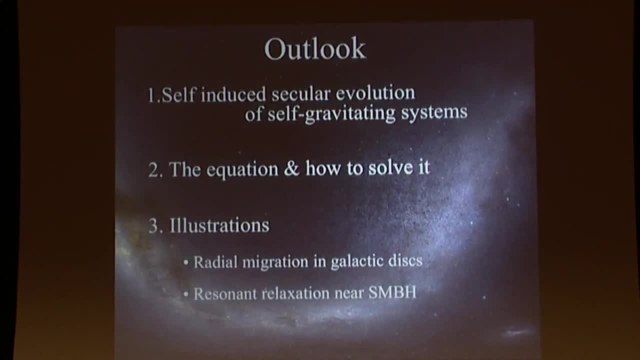 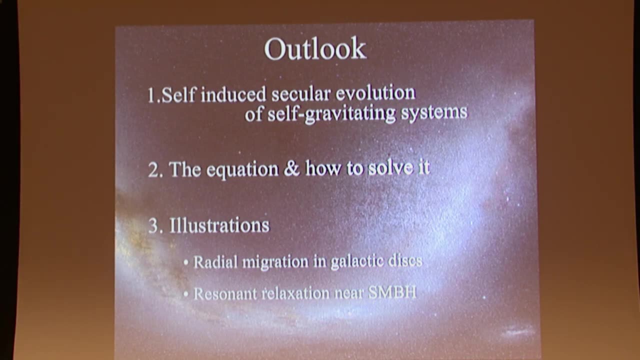 secular motion for the orbits in the vicinity of the black hole. okay, so let me recap. we want to understand secular evolution, the slow process by which fluctuations of self-gravitating system evolved towards more likely state. so I'll divide my presentation in three part. first I'll motivate secular 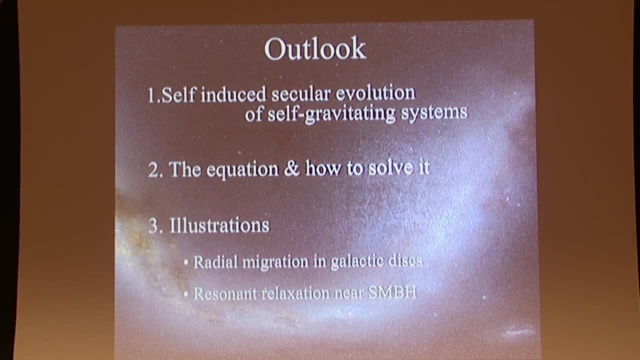 evolution, why secular evolution is relevant, and discuss the key physical features involved when one wants to describe the long-term evolution of self-gravitating system. this will be the core of my talk. then I'll present to you the corresponding equation that you've already seen briefly and discuss it and I'll illustrate it on two example other. 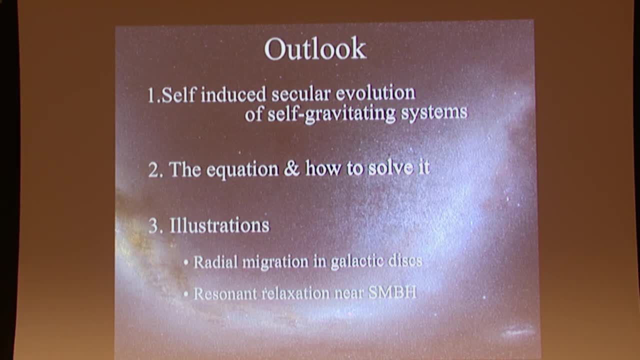 the issue of radial migration in galactic discs as a proof of concept, with quantitative comparisons, with simulations, and then I'll end up with the focus of what's of interest to this audience, which is the secular evolution of a quasi-keplerian system, and see how this corresponds to a 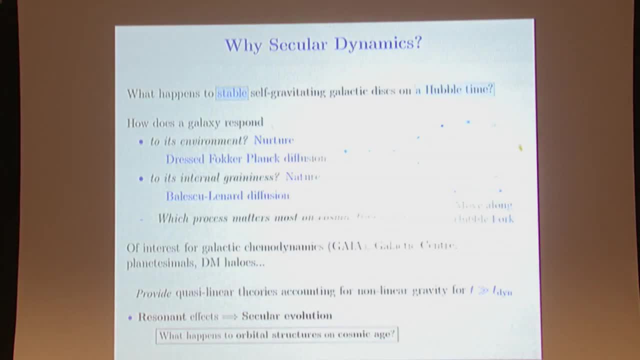 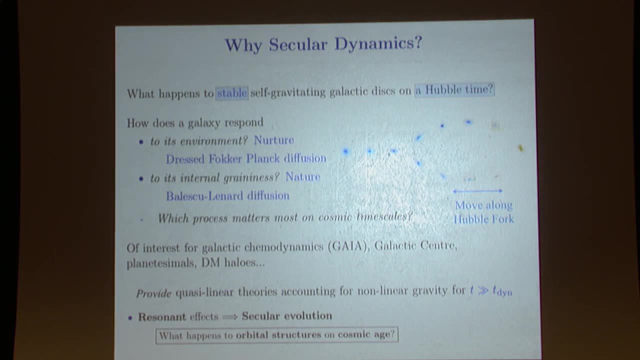 degenerate case of the general theory. so in this talk, we're concerned with understanding how stable self-gravitating system responds over long time scales, and so one question we may ask is: how can a galaxy evolve along the Hubble sequence through its self interaction? so we had, in the process of 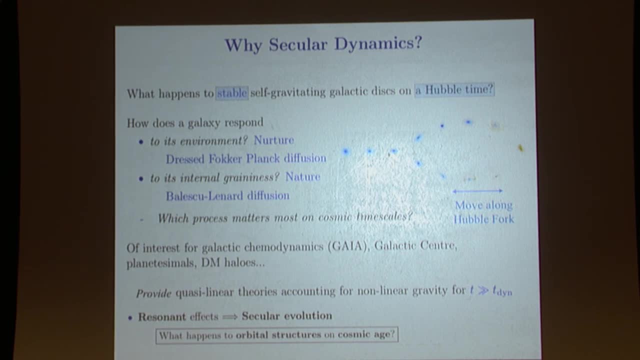 trying to disentangle nature and nurture, and nature being its internal driven evolution, and nurture being eternal space, evolution which we'll discuss later, nurture being the impact of its cosmic environment. And so I'll focus on, I guess, nature in this talk. 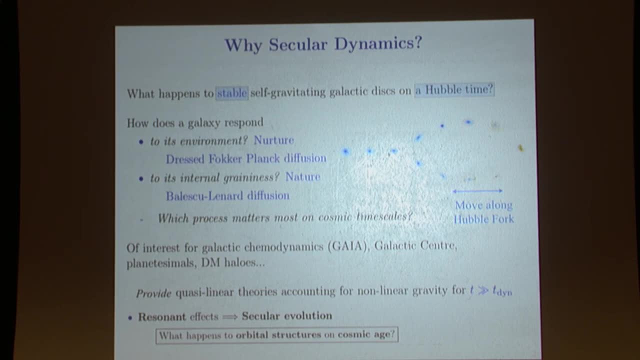 And the motivation is chemodynamics, et cetera, And so our task is to build the corresponding quasi-linear theory, which should be valid for timescales which are much longer than a typical dynamical timescale, And, as we will see, the secular evolution will be driven by resonant effects. 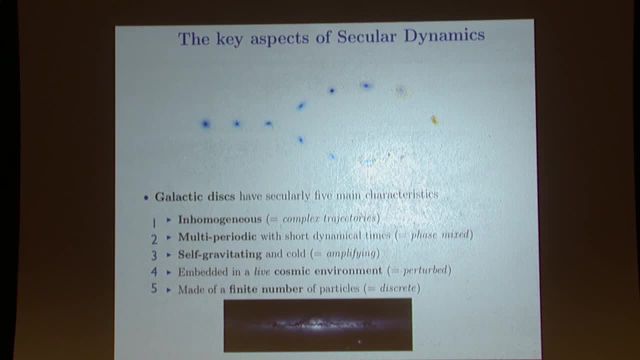 which distort the orbital structure. So basically, the five points I want to make in this first part of my talk is that galactic disks have specific features which are relevant for long timescales. They're inhomogeneous, as mentioned already by Pierre-Henri. 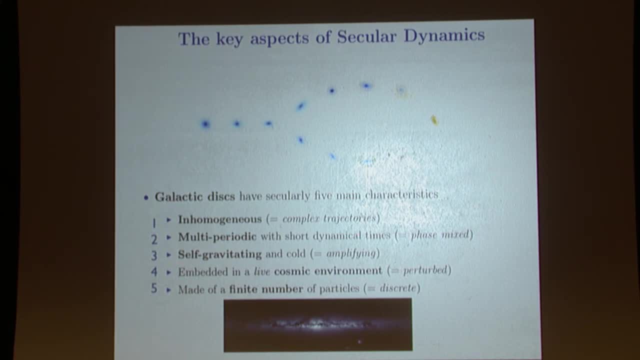 They're multi-periodic and phase-mixed, They're self-gravitational- And this will be a very important point for disks and also for the galactic center, as I will try to argue- And they can be embedded in a cosmic environment. 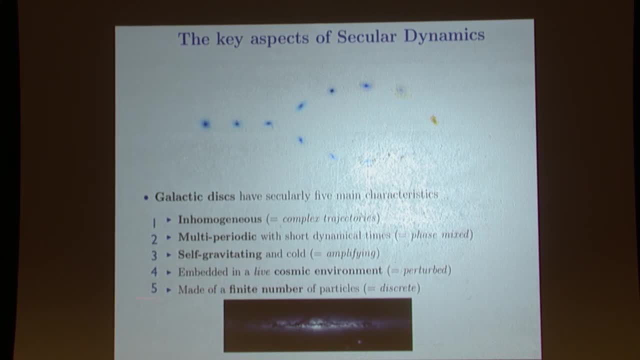 And they're made of a finite number of particles. This is true both for disks, where you have GMCs, but also in the context of the galactic center, where you have a finite number of stars orbiting the black hole, the central black hole. 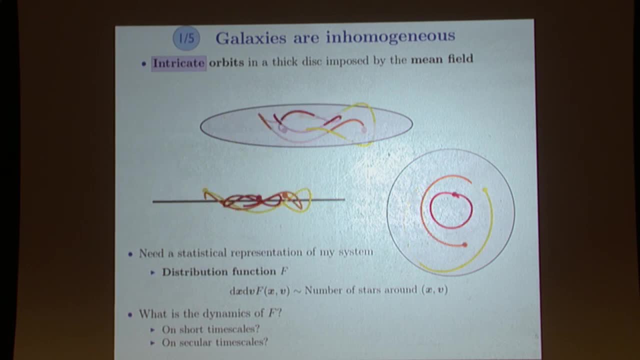 So the typical trajectories of stars in a galactic disk are quite intricate, And so, in order to understand how the self-interaction of such stars, describing their orbit, can drive the orbital structure of the system away from its state of equilibrium, we need to have a statistical approach. 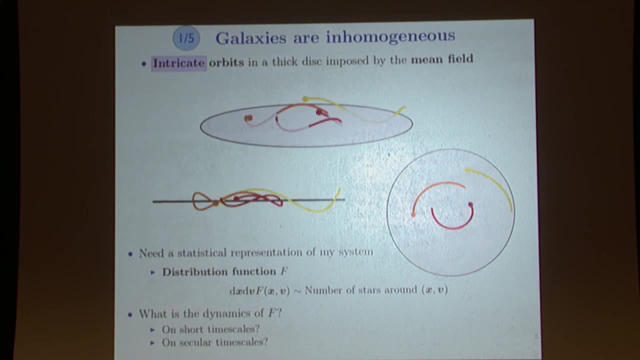 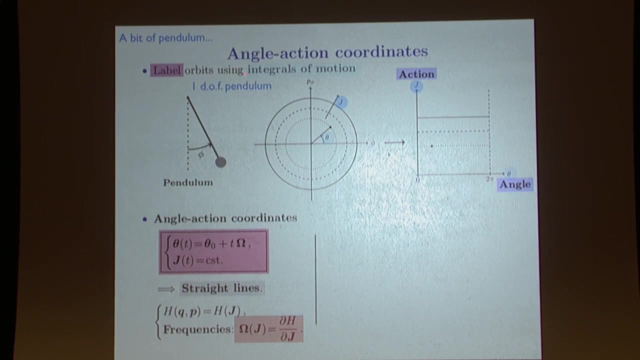 and look at the evolution of the distribution function, And so we need to make sense of these complicated trajectories. So this can be done by introducing so-called angle-action coordinates, which are, in some sense, for those of you familiar with Delaunay variables. 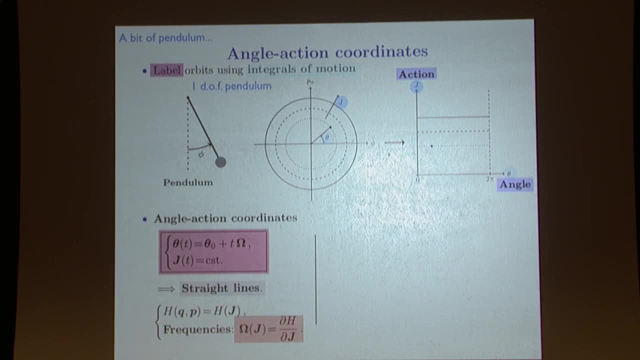 are a sort of generalization, in the context of galactic dynamics, of Delaunay variables. So, taking the example of a pendulum, if we want to describe the dynamics of a linearized pendulum in configuration space, we're better off moving to phase space. 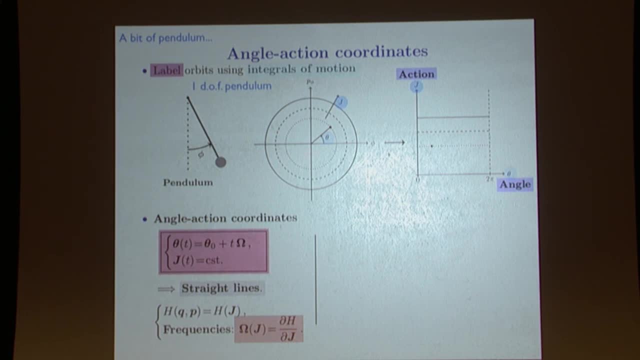 where, basically in phase space, the trajectory is labeled as a linearized pendulum. So this is represented by the area of the trajectory in phase space and the position of the pendulum is represented by the angle. So if I use these new canonical coordinates, 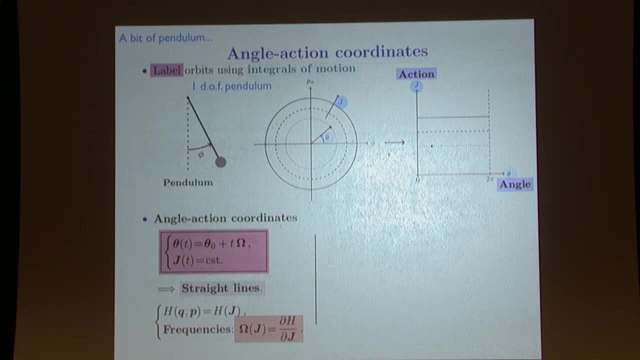 as a representation of my system, then, because the area is a constant of the motion, the Hamilton's equation trivially becomes straight line in angle-action space, And so this allows me basically to recover the uniform medium description that Pierre-Henri has been describing previously. 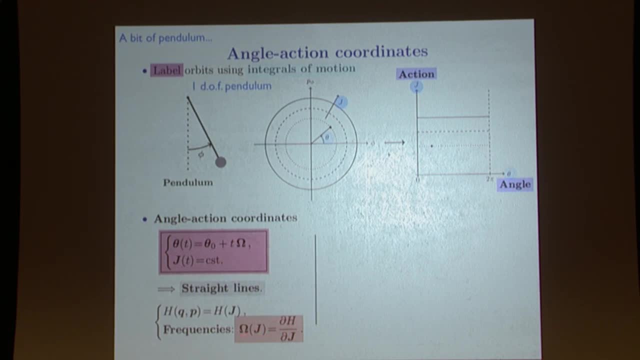 And so it enlightens also the specific role of the frequencies, which are just simply the derivative of the Hamiltonian, with respect to the actions And something. so it's rather boring in 1D, but something quite interesting happens if you consider a 2D pendulum. 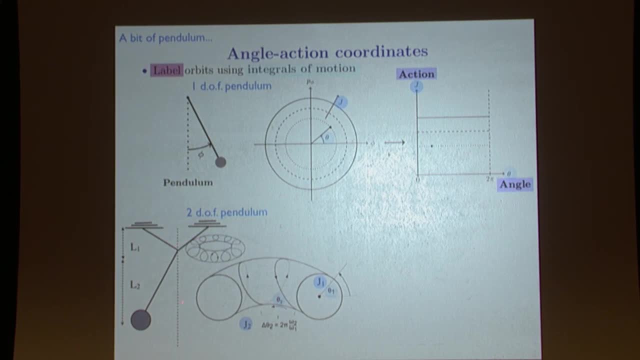 so two strings attached together in a one-cycle string. So this linear 2D oscillator will be a 2D oscillator and it will behave like the direct product of two 1D oscillators, And so in phase space, the typical trajectory of the pendulum. 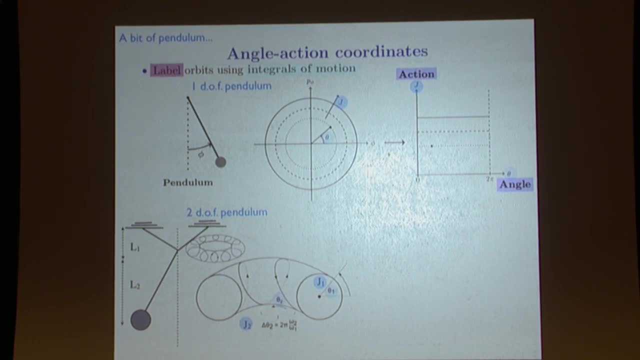 will be a trajectory along a torus, And one of two things can happen, depending on the length of the strings of your pendulum. Either it leads to frequencies which are commensurate, so there's an integer number relating the two frequencies, in which case the trajectories will describe. 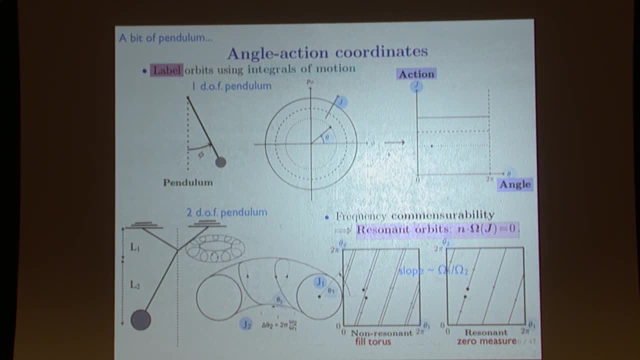 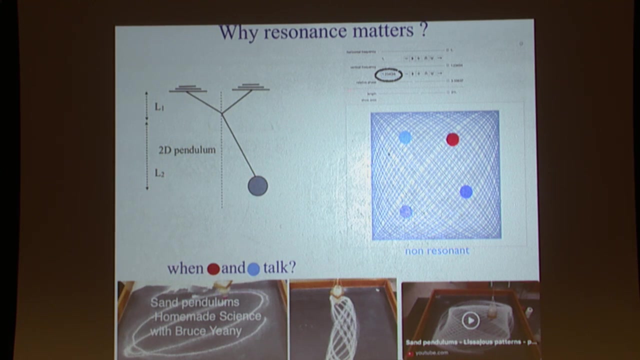 a trajectory of zero measure on the torii, or they're non-resonant, and then the trajectory will fill the torus, And so you see that from the point of view of recurrence this makes a big difference. So if I choose two frequencies, 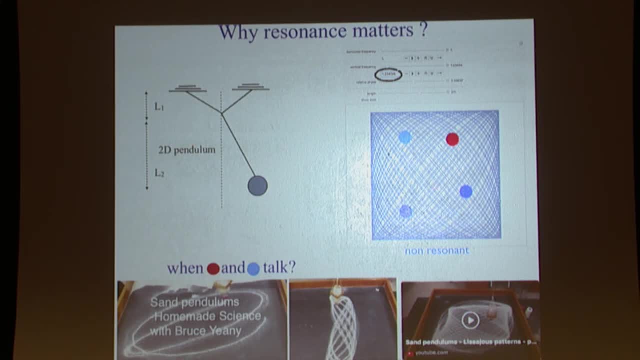 which are not commensurate here on this 2D pendulum. and I ask myself: how often do the blue particle meet the red particle When they're not resonant? it happens quite rarely, Whereas, conversely, if I consider the situation, 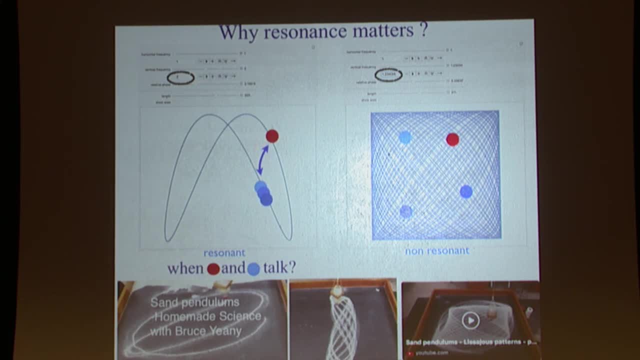 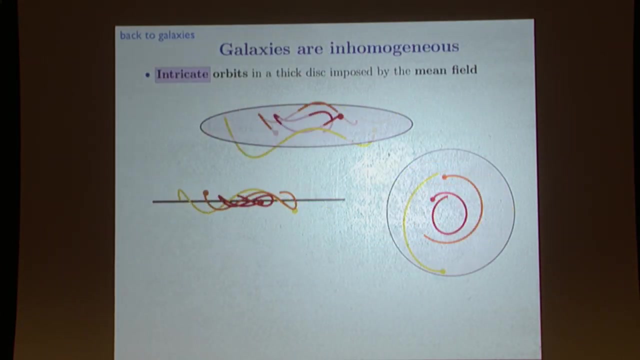 where there's a commensurability, then the likelihood of having a recurrent meeting between the blue and the red particle augments considerably. So you see why recurrence is driven by resonance, which is driven itself by the natural frequency of the system. So if I use this action back to 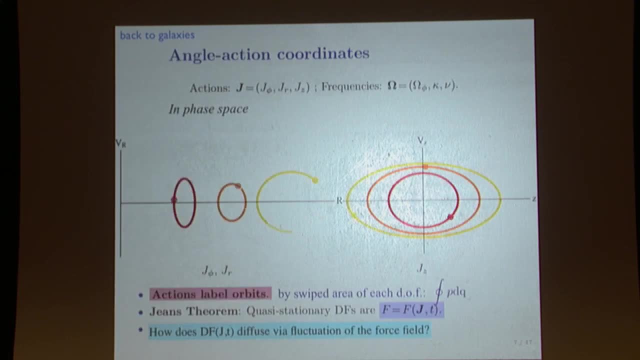 this angle-action variable back on my galaxy, then I, by going to phase space, I can see they can easily label the orbits using these, these actions. um, this is VR versus R and V, Z versus Z in phase space. and so then the question of how does the distribution function of my system? 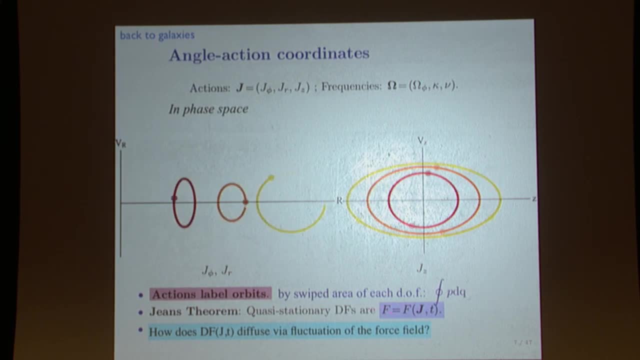 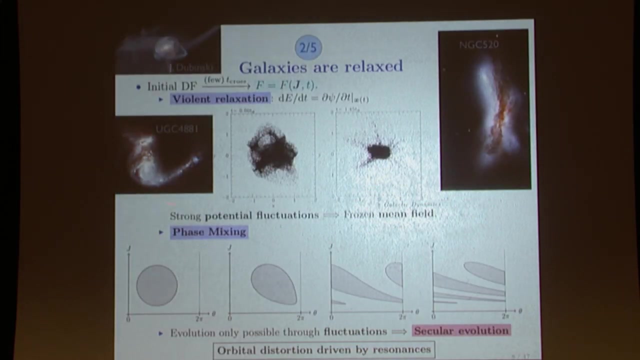 evolve with cosmic timer becomes a function question of how do these action get distorted by the diffusion process? and so the? the answer is through dressed, resonant interaction, which is what we're going to see. so let me move a bit more quickly on the more trivial points I want to raise. so galaxies are relaxed. 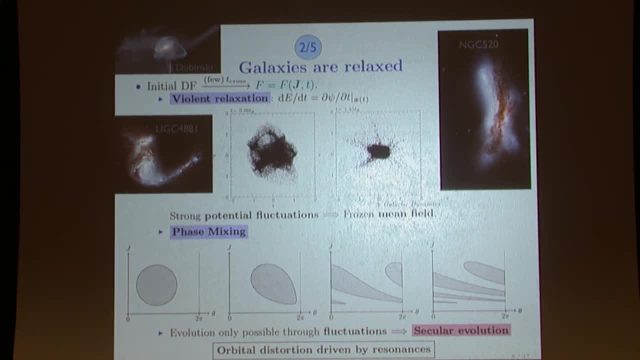 everybody knows that first through violent relaxation the potential becomes time independent and then through phase mixing, the distribution function loses track of its angle and depend only on the actions. so we're really interested in writing an equation for the evolution of the distribution function as a function of action. 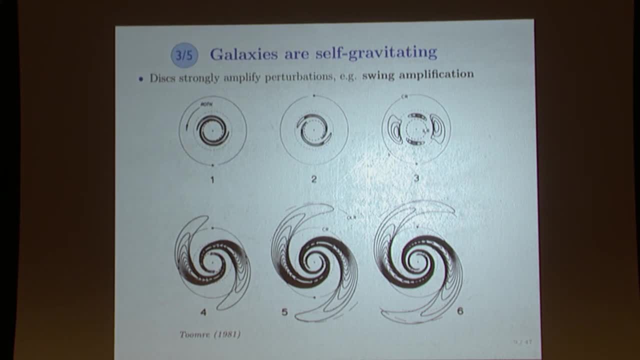 only galaxies are self-gravitating, which means that you have a leading spiral and I let it unwind. it will be strongly amplified by a factor of more than 100 for a Mestel type disk and this will play a key role in in secular evolution, because this amplification will be squared. 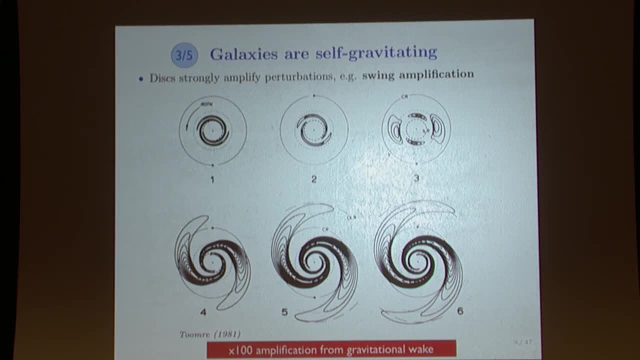 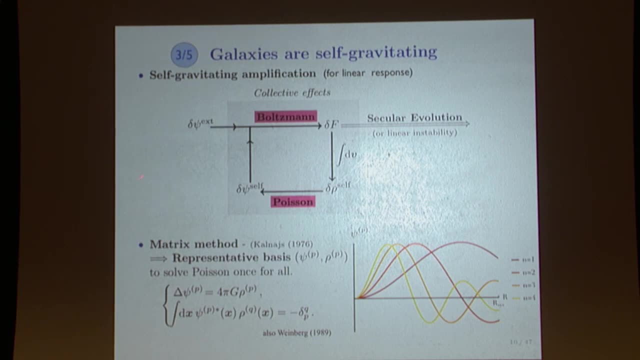 Jean-Pierre Henry already mentioned the fact that the, the gravitational susceptibility, is squared in diffusion equations, so you get a factor of 10,000 places per second at a given time. here we have a bevel out, here is a positive degree of force, of force on one side, and we can take necessary responses as 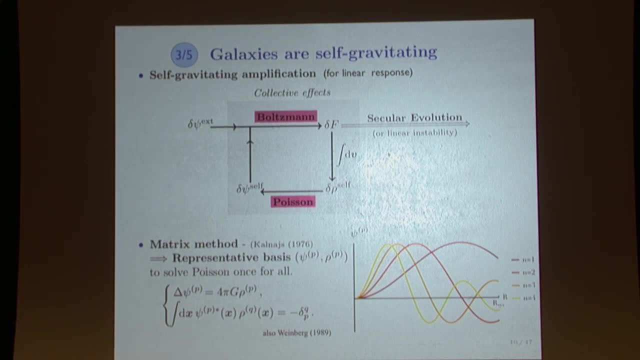 well as the time-dependent coefficients. so the way you deal technically with disamplification is by using a potential density basis introduced by Carlise. so you you basically make the field equation disappear by projecting the response of the system over a basis which automatically satisfies Poisson's. 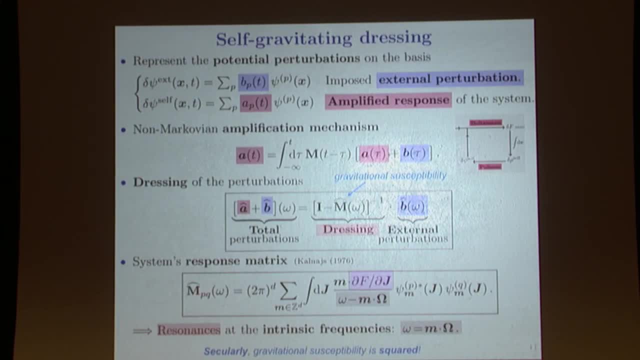 equation. so by magic you don't have Poisson's equation anymore. the price, you the details. it involved this matrix, response matrix introduced by Carlisle, which involves this resonant denominator, again, the relevance of the resonance in this problem and, importantly, the the gravitational wake of the gravitational. 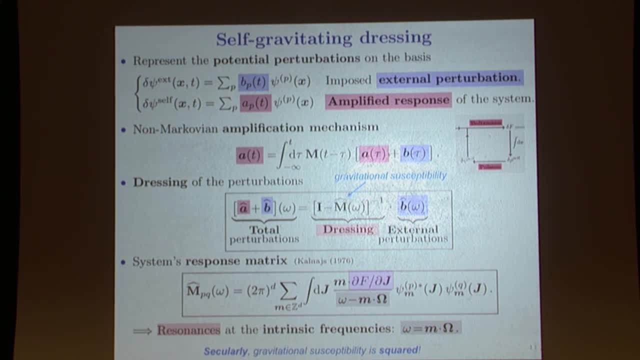 susceptibility involves the inverse of this matrix response. so when it has a one as an eigenvalue, you see that the system can amplify exponentially its perturbation. so in the context of secular evolution we assume it's not the case, but it can be close to one, so the amplification can be quite strong. galaxy. 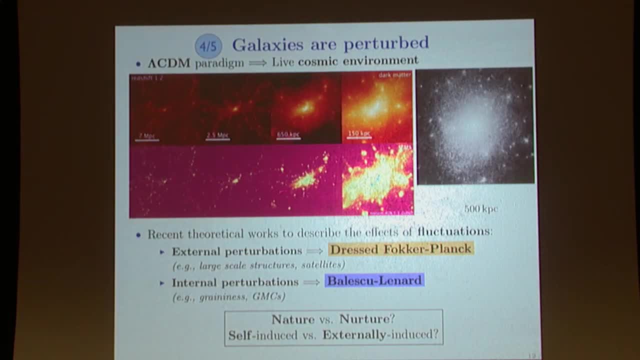 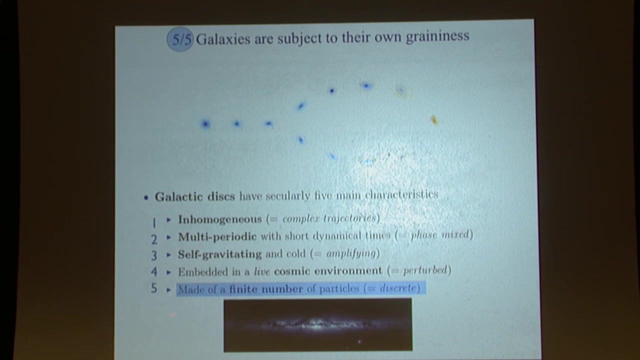 of the tub, so they're embedded into a cosmic environment which is going to act as a source of potential fluctuations which can also drive diffusion- but I guess this will not be the topic of this talk- and galaxies are subject to their own graininess. so as, as piano, he has shown you the, the. 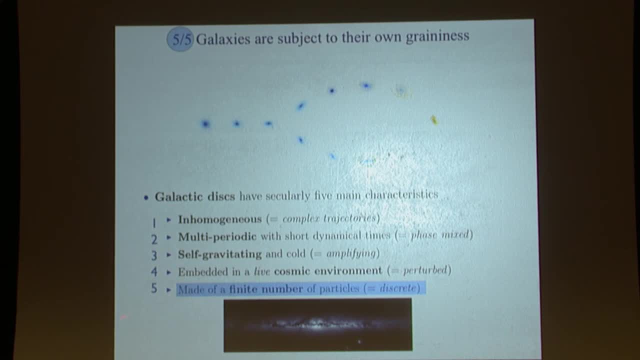 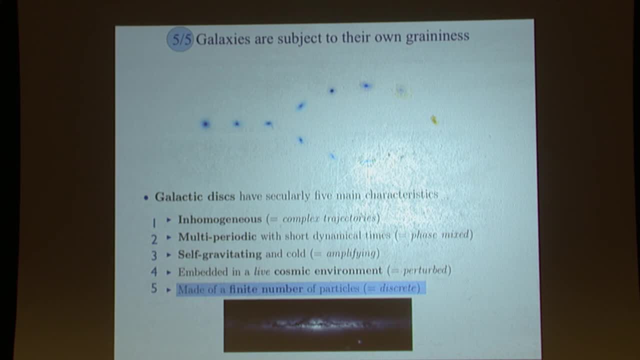 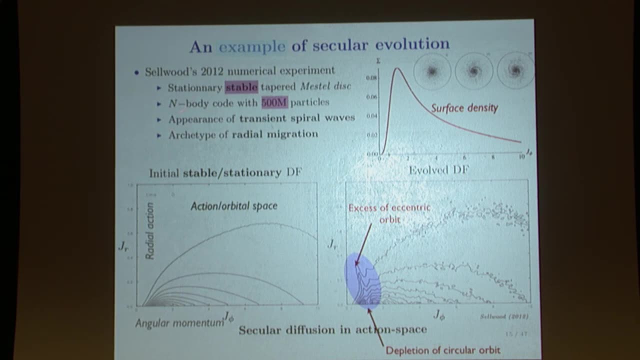 from the mean field-limit. if you've got an infinite number of stars, this term is zero. but here we're interested in finance system made of a finite number of particles. okay, so let me give you an example. to be more concrete, this is a numerical experiment done by Jerry Selwood in in. 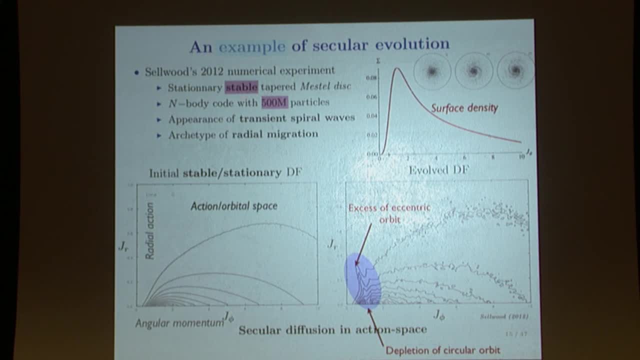 considers a built to be stable Mestel disk with half a billion particle and he lets it evolve over many dynamical time, And so this is the initial configuration in action space. So you have an excess of stars corresponding to this surface density here. 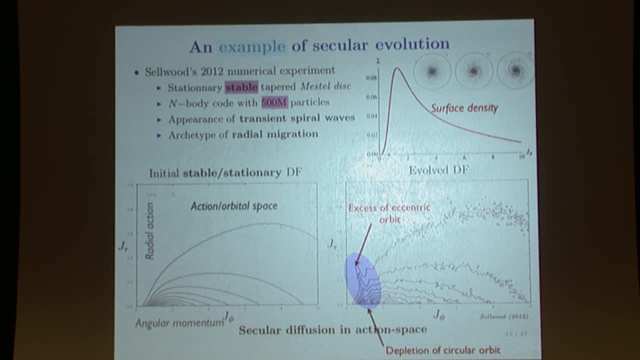 and this is not working anymore. And after many dynamical time, you see this feature which is emerging spontaneously within the system, Even though it was built to be stable. so in principle, nothing should happen. So you see an appearance of an excess of eccentric orbit. 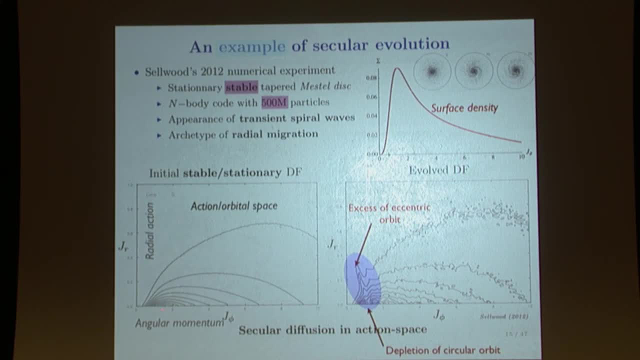 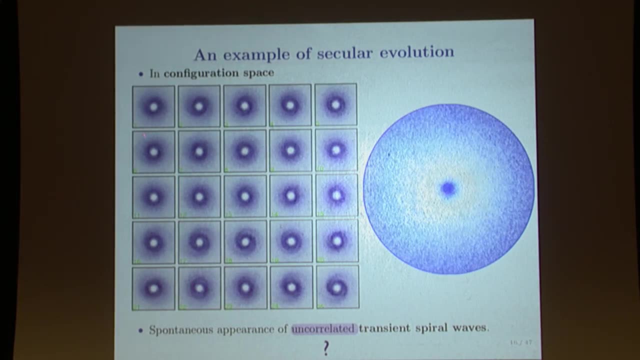 and a depletion of circular orbits in the vicinity of the maximum of the distribution function in action space. So this is secular evolution. If you look at configuration space- this is us reproducing this experiment- you see that nothing is happening at all. The disk is just happily rotating. 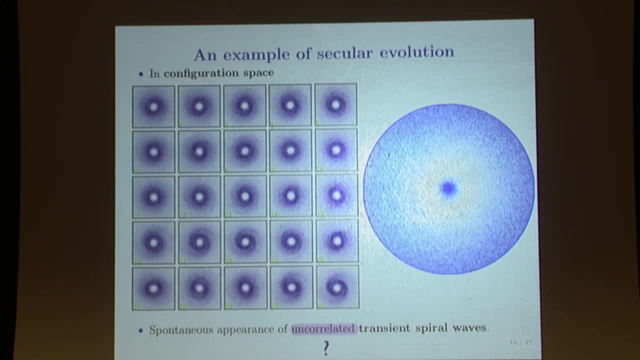 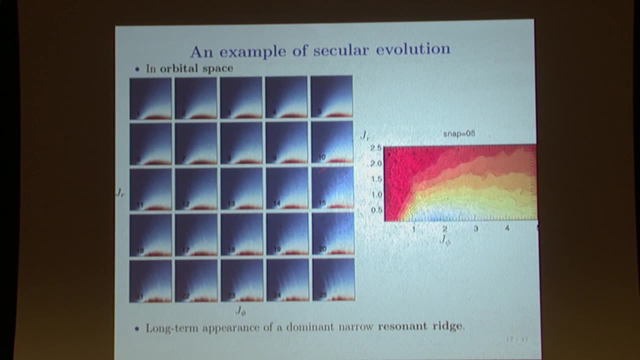 and forming weak transient spiral which disappears. But if you move to angle action space, you see with this animation that I don't know how to slow down, So every time it runs it's a Hubble time. So and you see the appearance of this ridge. 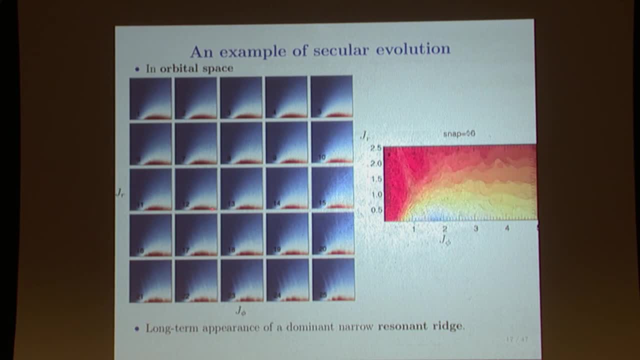 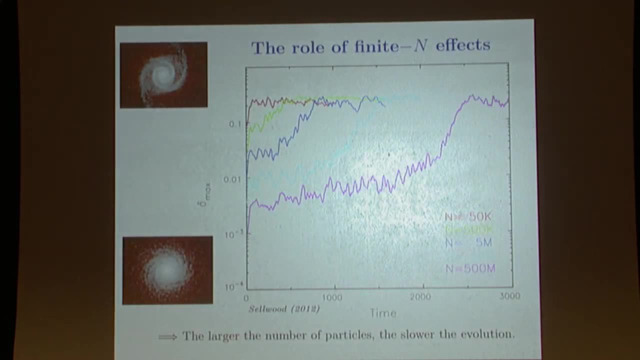 which can be seen also on this static representation of action space. So secular evolution is about the distortion of the orbits induced by their self interaction, And this is a one over N effect, as shown by Selwood again, because if you increase the number of orbits, 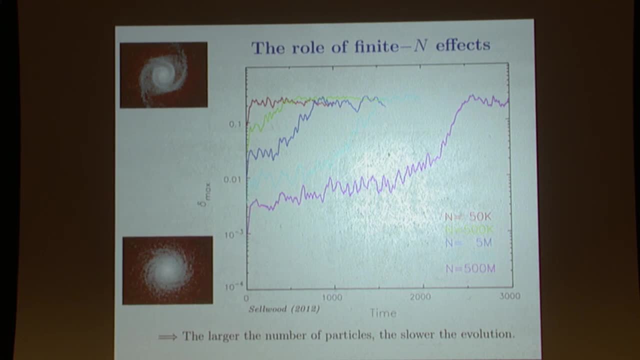 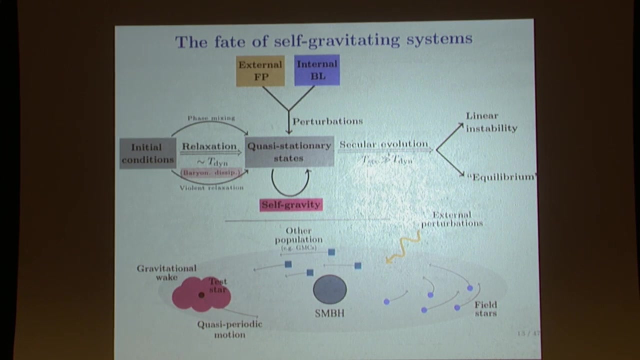 if you increase the number of particles in the run, you see that the time it takes for this ridge to appear goes like one over N. So Why not? Well, it depends on N Depends what system you're looking at. Yes, 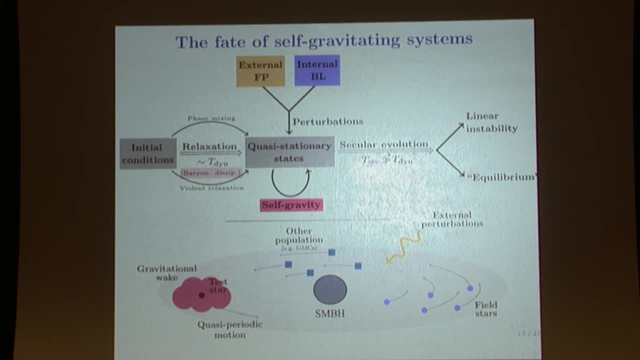 Yes, And the galactic center and is not one billion, for instance. So in Selwood's experiment, at the time it builds is commensurable the order of a Hubble time. but this was meant to be an abstract experiment. So in the real case it depends what. 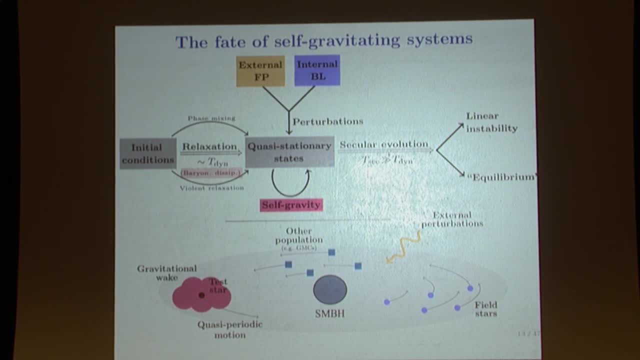 N is, if it's, the number of molecular cloud in the system. Because of the factor of 10,000 I'm talking about, it will grow much faster than what you would expect, would naively think. yes, then I agree with you, so so this is a cartoon of 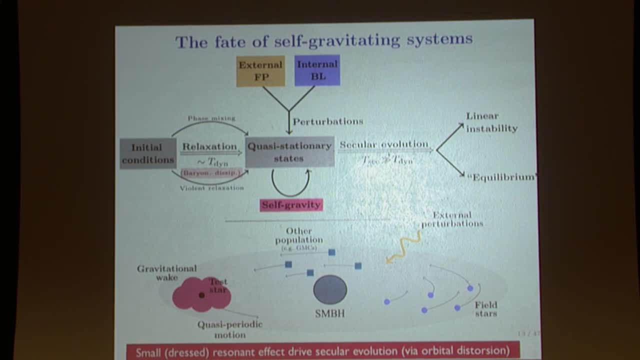 what's happening? you have your initial condition: violent relaxation. you reach a crazy stationary state and, depending on on the properties of the the system and the number of particles, they can evolve towards either an unstable regime or to a new equilibrium through secular evolution. okay, so let me just present to 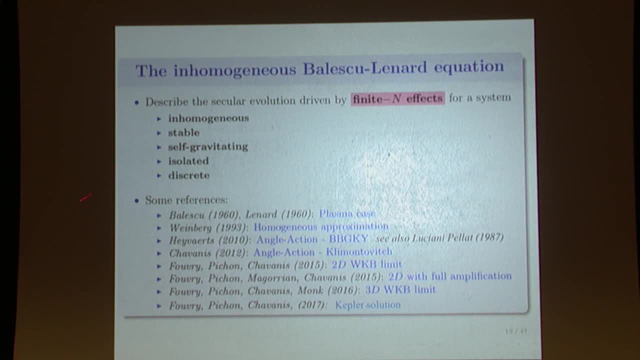 you the equation. I won't spend much time because it's already been done in part by a theory. it's supposed to describe finite n effects on long-term evolution of self-gravitating system which are inhomogeneous, stable, self-gravitating, isolated and discrete. there's some literature. 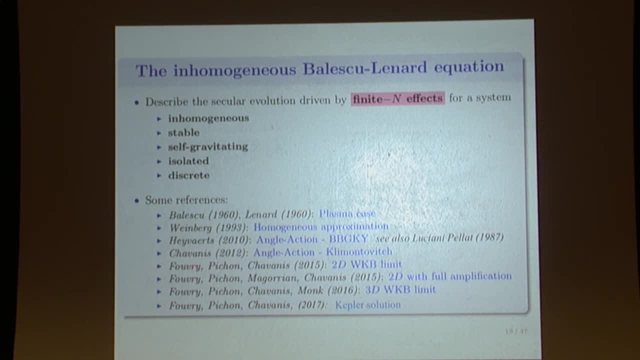 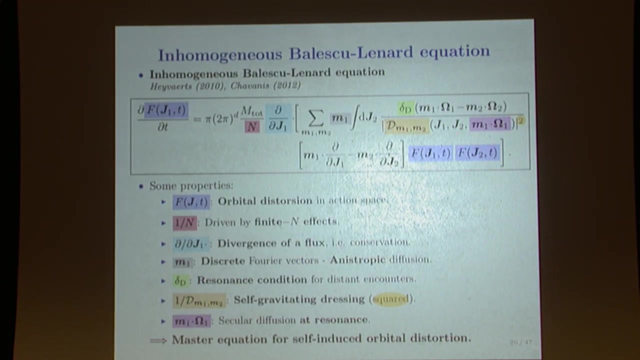 starting from Baliscou and Lennart in the 60s and I guess first first presentation was done by Jean Everts in 2010 and we and others have been working on it since. so this is the equation. it's an equation which involves. 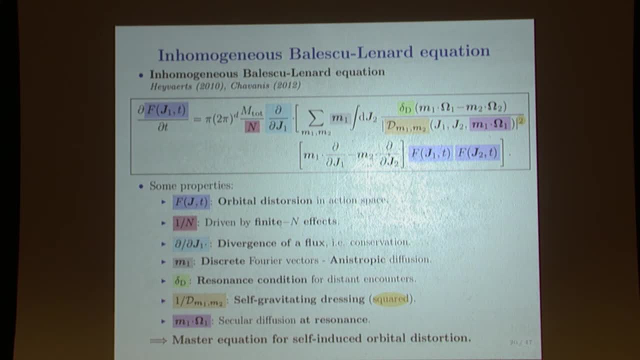 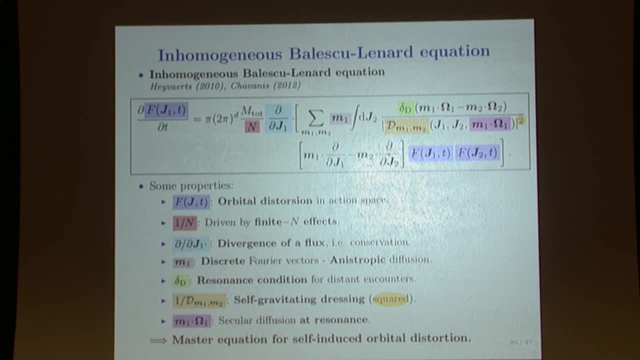 happen. these, these coincidences are amplified by 1 over the susceptibility of the. your gravitational system squared and you required that the stars involved are resonating and you some over all possible resonances. I'll come back to this. what else? yes, so you have these resonance condition and this is. 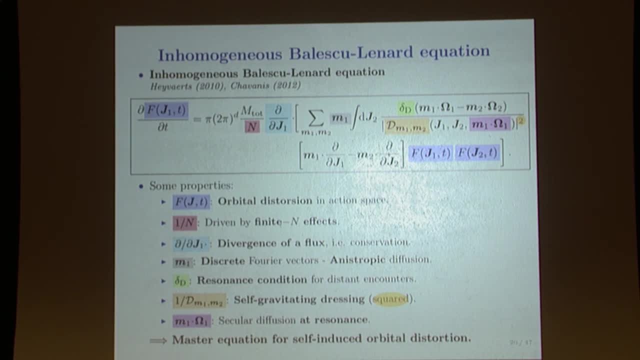 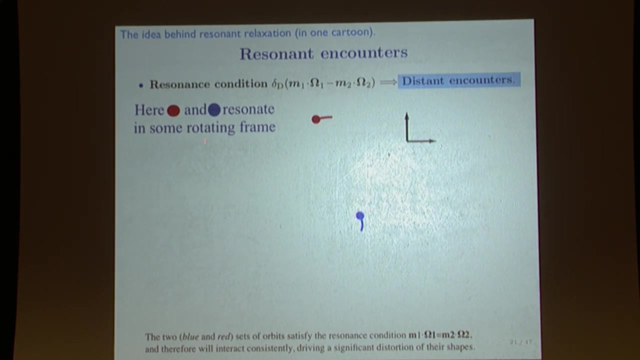 this is the master equation describing a self-induced orbital wave. but that's the orbital distortion, such as orbital relaxation, the paper by resonant relaxation. sorry, resonant relaxation. so the idea behind resonant relaxation is it comes from this condition of resonance that you have to impose. let's 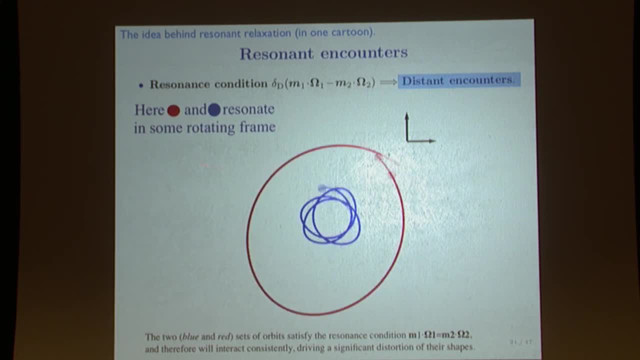 let's ask ourselves what star blue and red are doing and move to a co-rotating frame so that within that co-rotating frame both the blue and red orbits close, either as an indolent bladders or co-rotation resonance, and you. 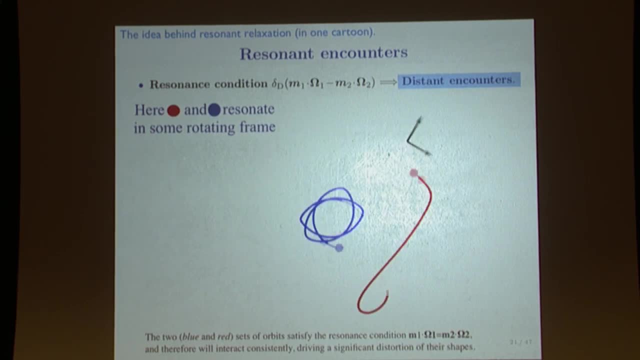 see that in this co-rotating frame they will be able to exchange some angular momentum and and in this process, restructure their, their actions. so this is this is what happens in the co-rotating frame: the two orbits satisfy the condition of resonance and in that frame they can exchange some. 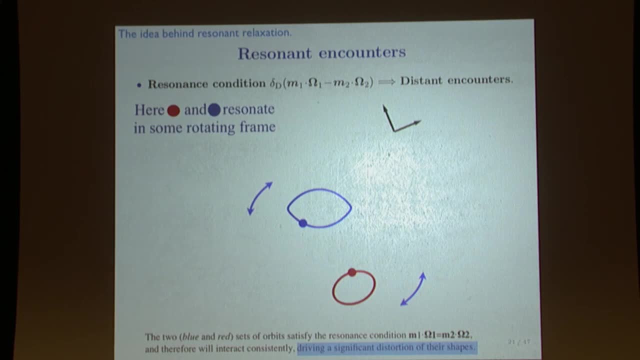 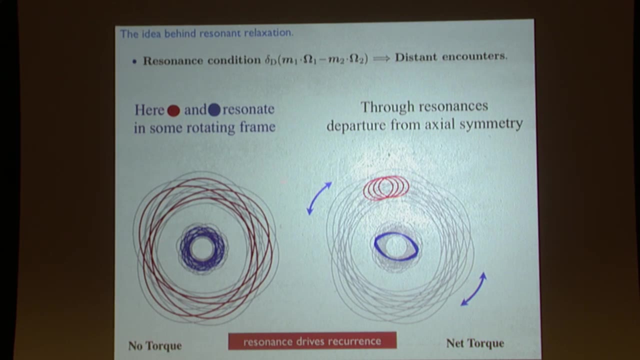 talk, and through talking they can change their actions and so allow the orbital structure of the system to diffuse. so this is another representation: if the two stars are not resonating, and then they don't exert any talk on each other because they're actually actually actually distributed, but if they do, 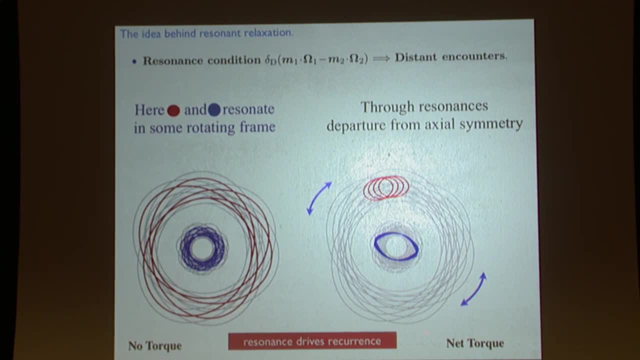 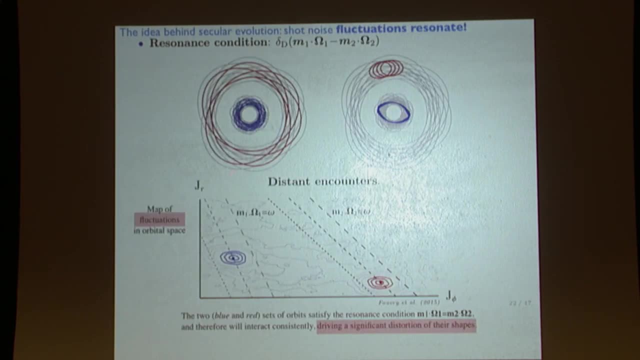 resonate, then they can apply. resonance apply some talk on each other, And so resonance drives the recurrence and drives the ability for the system to evolve. Now, if I focus specifically on fluctuation-driven evolution and I look at action space and I look at the distribution function, 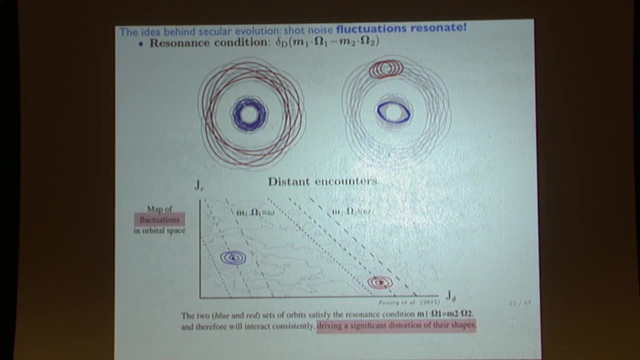 and its fluctuation at a given time. if the blue fluctuation happens to resonate with the red fluctuation, meaning that they are sitting on lines of constant m, dot, omega which match each other, then these fluctuation can gravitationally talk each other. 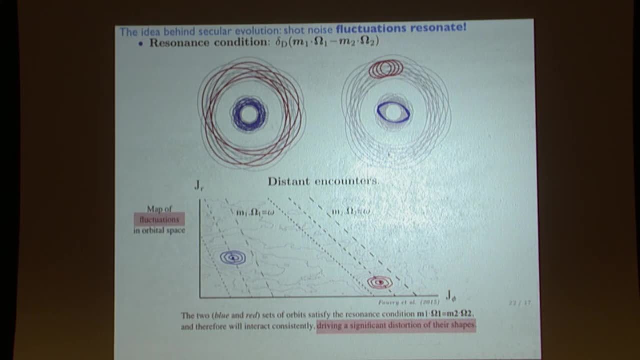 and amplify themself, And this is what's driving the secular evolution. Is that clear to everyone? Is this sort of clear? No, yes, maybe. So the coupling that can occur through this resonant condition allows this short noise perturbation to be gravitationally amplified. 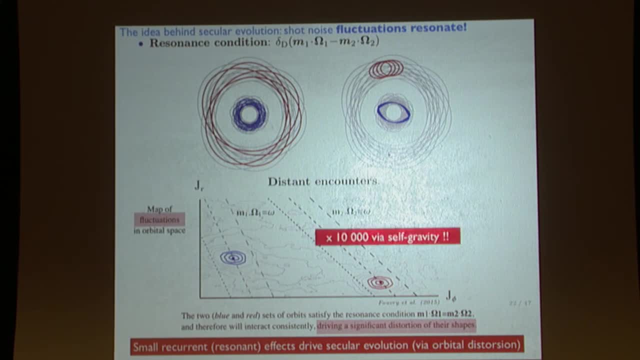 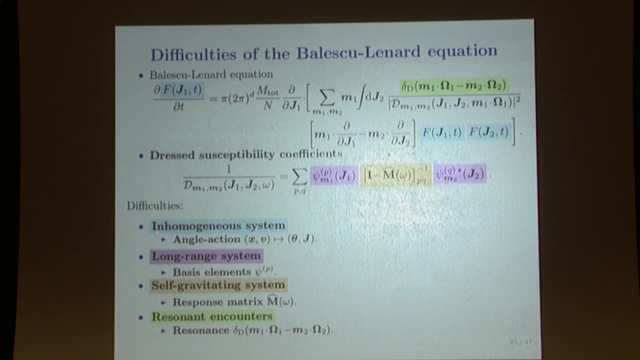 So it can be amplified by the square of the gravitational susceptibility. So for cold Mestel disk that would be a factor of 10,000.. Okay, so how do you deal with the actual implementation? Because it's one thing to write an equation. 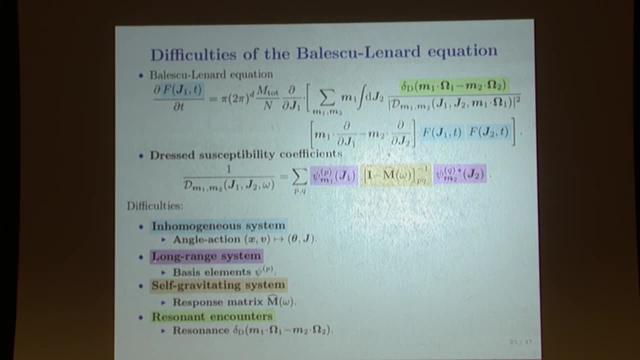 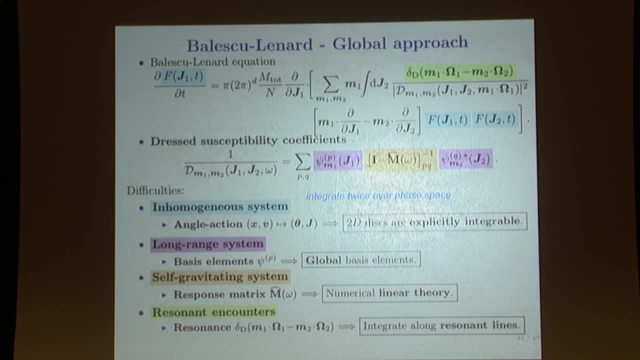 but then you actually need to implement it. So you have to deal with the fact that the system is inhomogeneous, long-range, self-gravitating, and you need to deal with these Diracs. So that's the hard part. So what you do is you use. 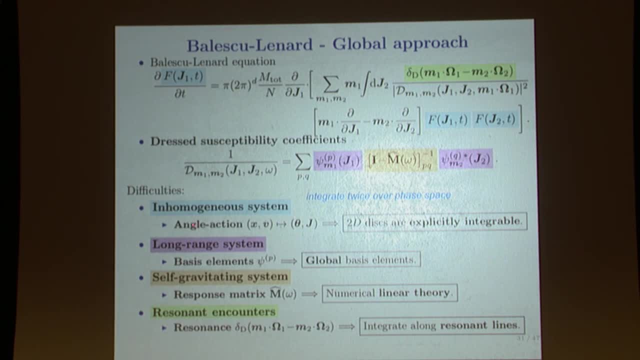 you use angle action to deal with the homogeneity. You project the Poisson equation over the basis function to deal with the long range. You use numerical linear theory to compute the matrix response- and that's a big piece of work- And you integrate along the resonant line. 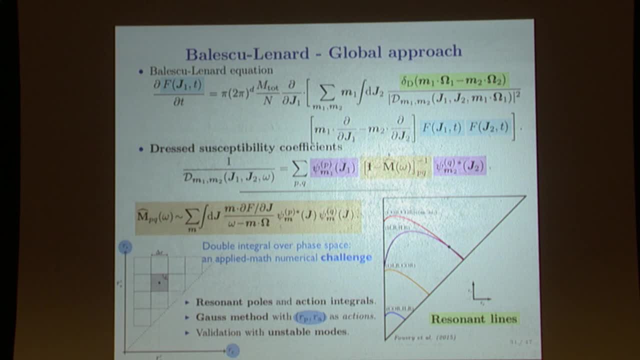 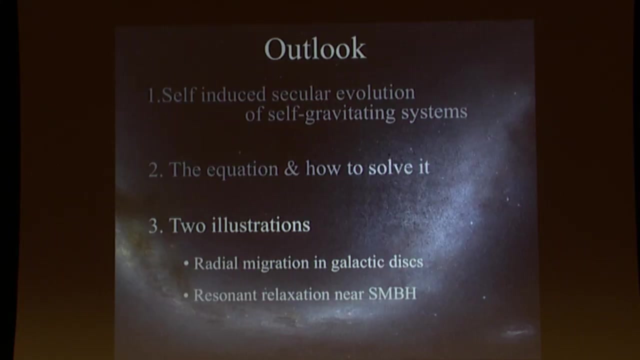 So I won't go into the details because it's technical and a bit boring, but you have to keep in mind that you need to integrate twice over phase space, so there's no free lunch, and that's where the the cost is going. but it's doable, and it was the topic of Jean-Baptiste's PhD, and so let me now 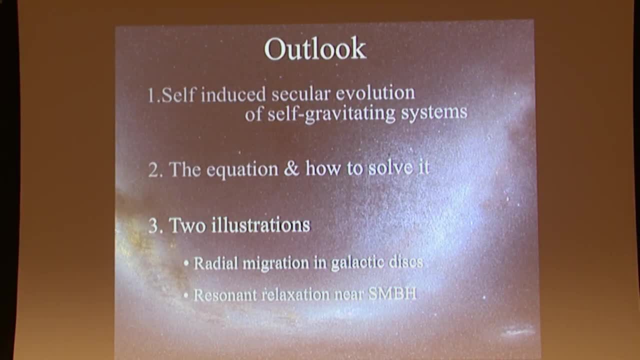 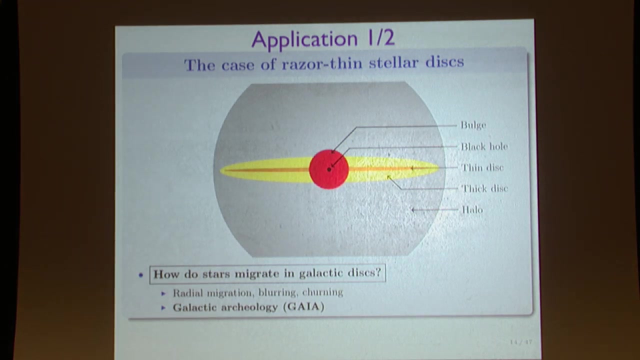 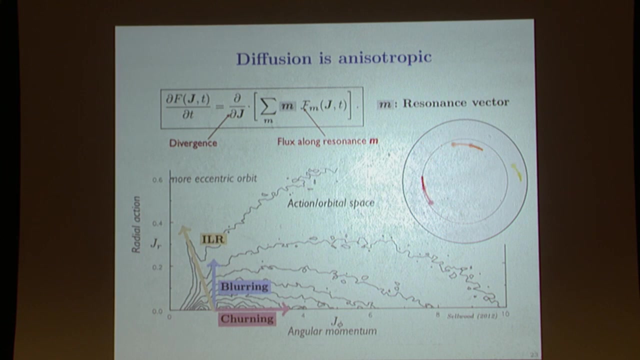 illustrate briefly how much time you have. okay, let me slow down, maybe it will be better for everyone. so let's move to the understanding. what happens to a, to the, the cold stellar disk. so the structure of the equation is is a diffusion equation, with a flux which involves the sum of a resonances. so this: 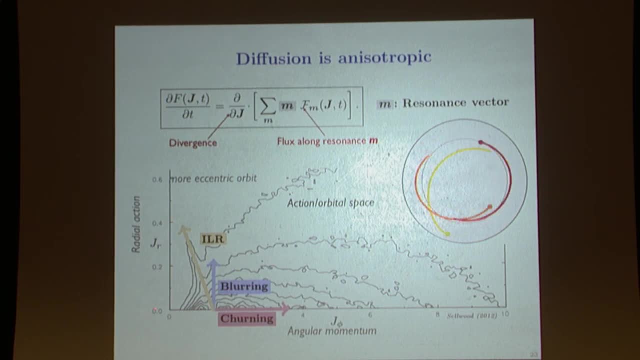 is sort of what which. what led us to to address this problem when we saw, when I saw the paper by Jerry Seward, that the fact that the ridge seems to be specifically along the inner Lindblad resonance suggested that it must be a resonantly driven process. 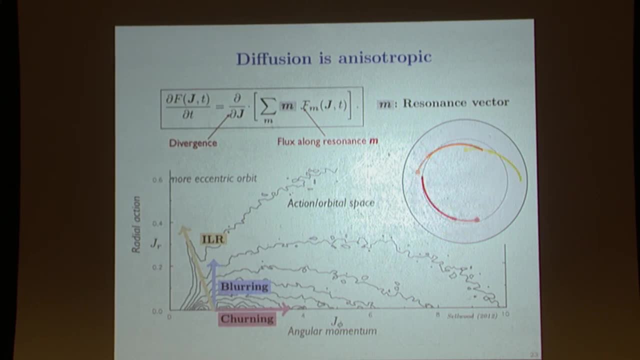 which is responsible for the secular evolution. so what you see here is that these, the stars which were initially here, are going to be the inner Lindblad resonance with itself. there's no there, with the excess of orbits in this area, which allows them to communicate by inner Lindblad resonance. 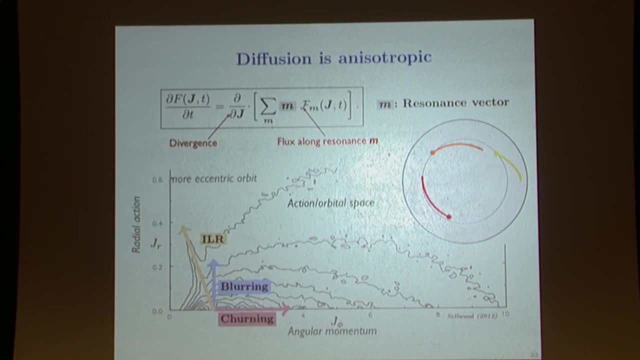 in the case of our galaxy, it is as far along as we can go. it's a good question and there's a good answer, but I'm really jet-lagged. so give me, let me think, but, but you don't have to have something to resonate, sorry. 12. 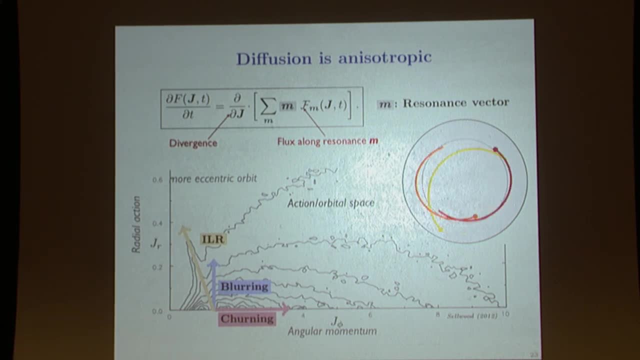 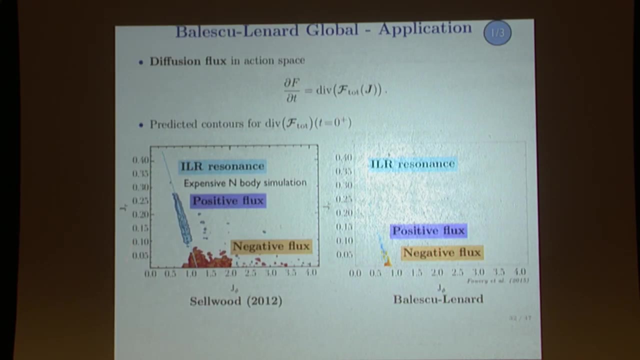 minutes. yes, thank you. okay, so this is- this is a, again from Jerry Seward- a representation of the fact that you have a positive flux, that is a positive flux, which is, which is a very significant representation of what's happening in flux in this part of action space and the depletion here, and this is the 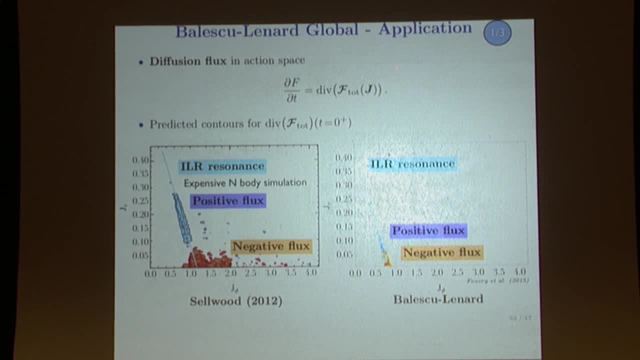 result of the Balis-Coulinard implementation where you compute the, the divergence of the, the flux, through the matrix response. so you see that, qualitatively at least, and to some extent quantitatively, you do recover, through the formalism, the fact that you have diffusion along the the correct. 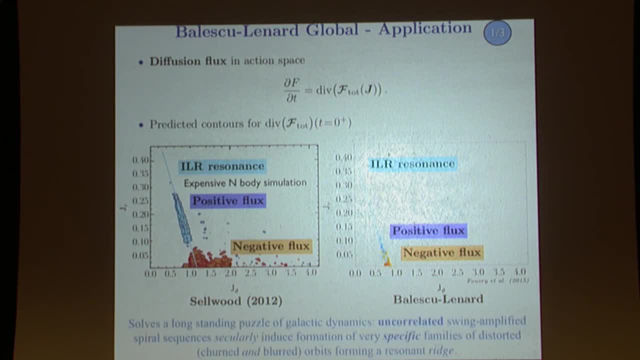 Ridge, the. so this, this solves a long-standing puzzle in galactic dynamics, because for a long time people had been climbing that it was a sequence of swing-amplified response which was generating a ridge, which it's up with figuring the next sequence of swing amplified spirals, and that was the ongoing process. what we show here and 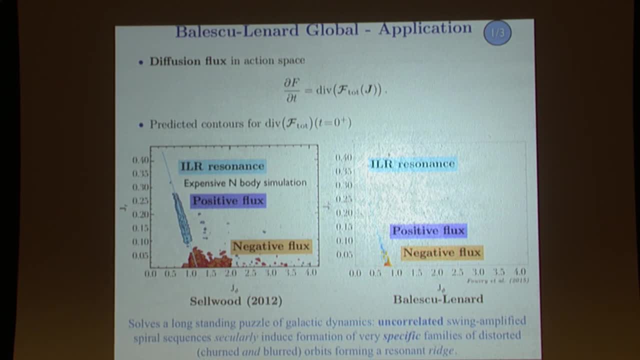 what has been also shown independently by Jerry's. this can't be the case, because the formalism assumes that the swing amplification are de-correlated, so that in the, in the baliscoulinard formalism, there's no, there's no correlation between the the swing. 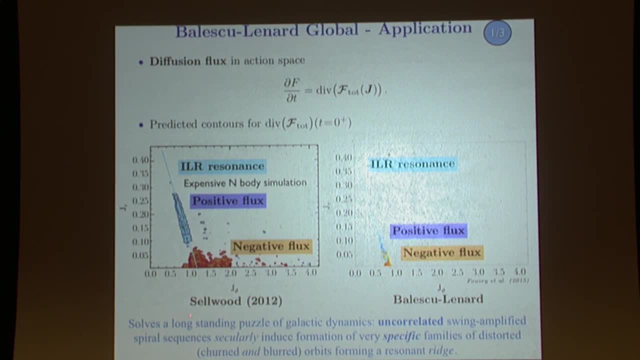 amplified response. and Jerry has also reached this conclusion because in his experiment he, he, after each spiral amplification, he and azimuthally averaged the the disc in order to kill any correlation. if there was any, and he would still see the same growth structure of this region in action space. 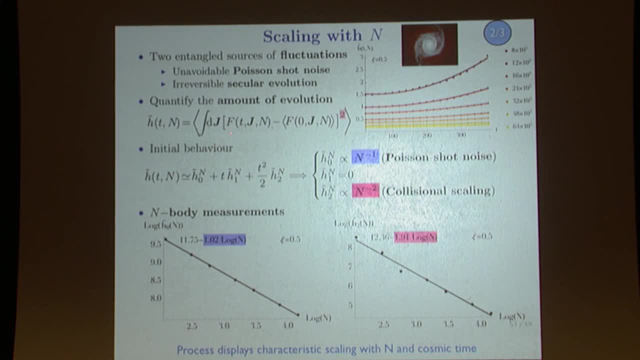 one thing we can do is check that the scaling we get as a function of the fluctuation and the scaling we get as a function of the fluctuation of the, of the distribution function, with both time and the number of particle, is consistent with one over n effect, so with the dissipation or flutation theorem. 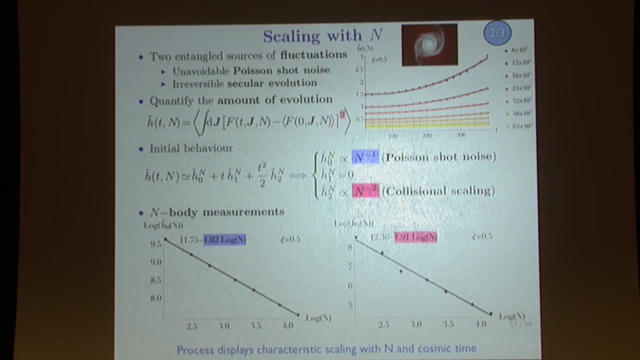 so we expand the, the, the variance of the flutation of the distribution function, and the theory tells you that you should have a contribution which goes like the initial shot noise and then one over n squared, coming from the collisional Ballets-Coulénard equation. and this is what you measure, so it's in good. 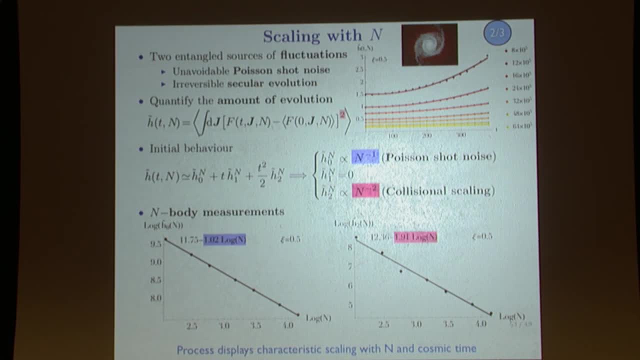 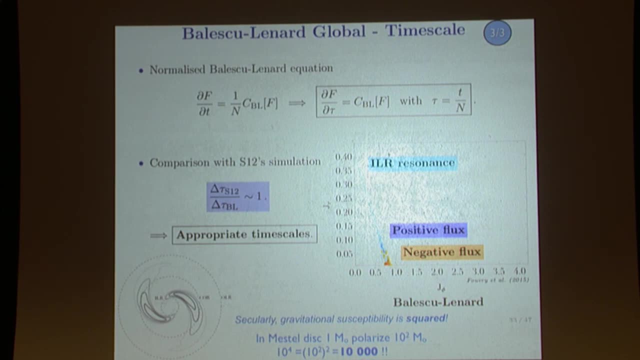 agreement. by doing many such such simulations and if you measure the time scale at which this perturbation builds up, the ridge grows into the disk. the Ballets-Coulénard calculation is also consistent within a with the words measured in the simulation, and this is thanks to this gravitational 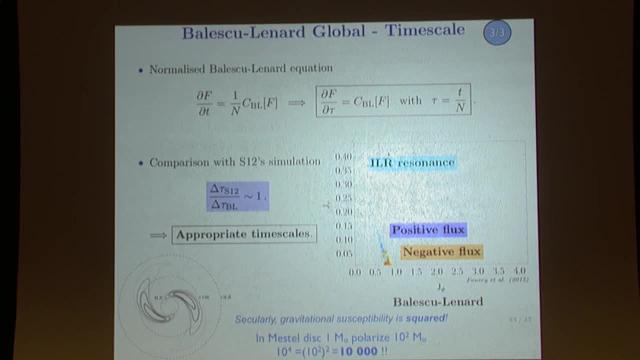 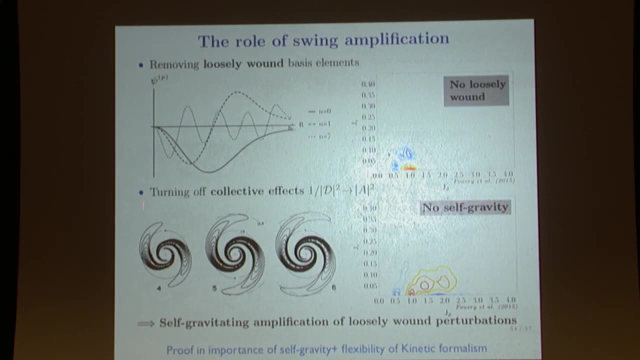 susceptibility, or the gravitational wake, which is squared in the equation, and you get a factor of 10,000 if you don't account for the gravitational amplification which you can do with such a semi-analytic system. so you can turn off the collective effects by just 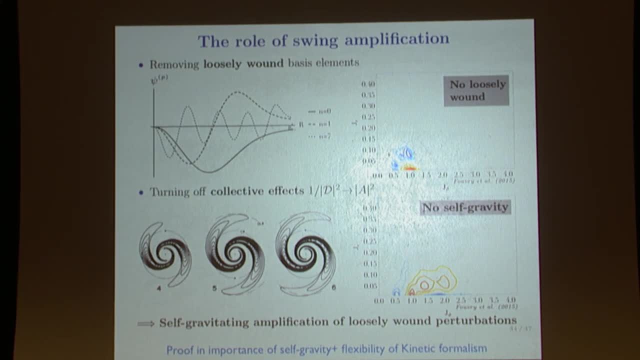 putting M to zero in the equations, then you see that you don't. you don't get the time scales and you don't develop the ridge. and similarly, you can convince yourself that it's truly the swing amplification process which is responsible for the, for the formation of the ridge, because if you kill in your 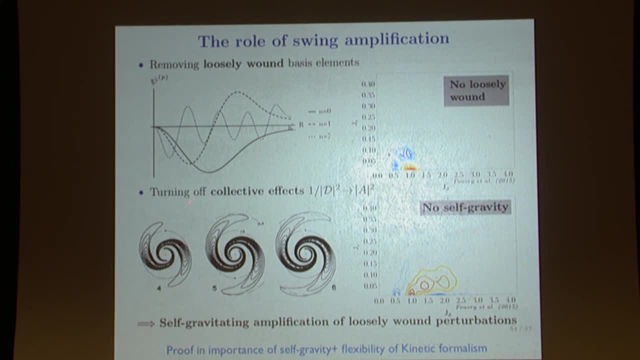 basis function, the, the, the unwind basis. so you only leave the WKB like basis, then you also kill the formation of the ridge. so I guess this I want to emphasize this is one of the nice thing about having a semi-analytical formalism- is you can play with these. 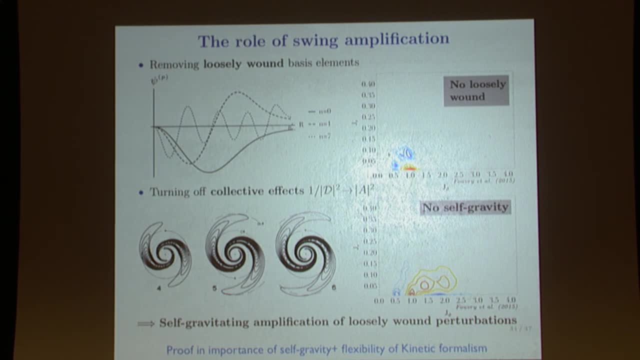 things. you can switch certain things off and see what what it does, which is much more difficult in the context of an N-body code. yes, yes, this is the second thought, this one. I want you to see that you don't have a nice ridge, it's, it's essentially noise. 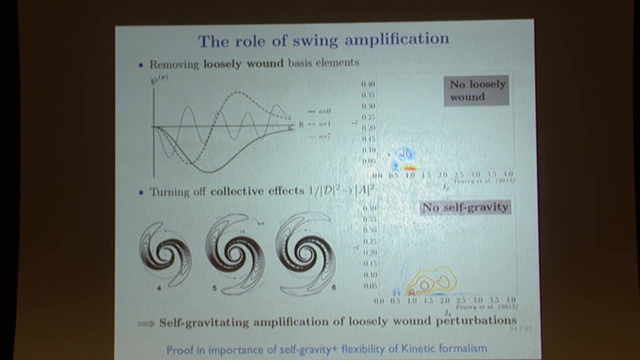 it's, it's small amplitude and it doesn't have the right timescale. you're getting the well have a few slides where we did this, the WKB with a WKB approach. so that would be exactly this and I can. I can show you later. it's you don't get to if you have. 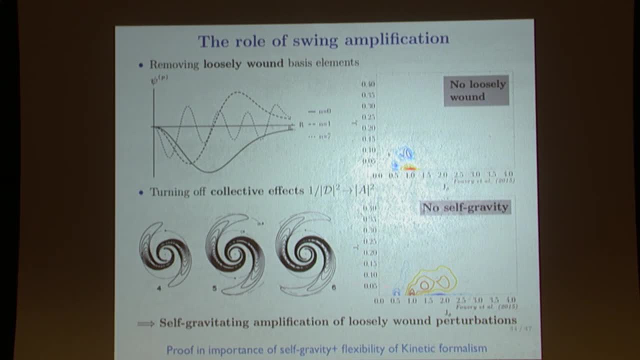 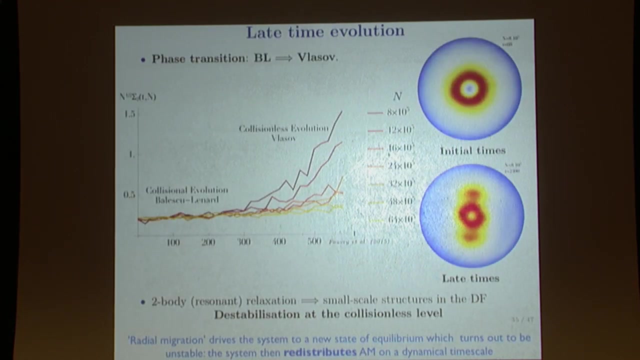 only WKB basis, then you won't get a nice sharp ridge. you get a depletion and an excess of eccentric orbits, but not at the roughly in the right region. so it's capturing some of the process, but not the right amplitude and the right sharpness and not the right timescale as well. what's interesting and also 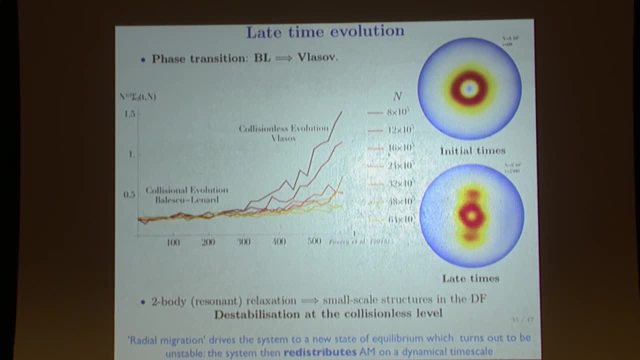 noticed by Selwood is that if you let this system long enough, it will actually do something. unexpected is, after a long secular timescale it will actually start to grow exponentially again if you look at the fluctuations. so the system has actually used the fact that orbits can. 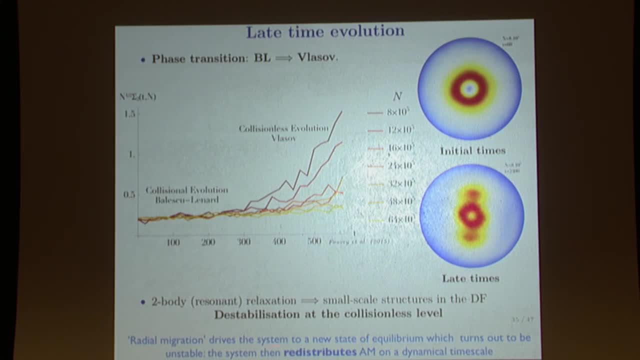 resit to the surface if you look at the fluctuations. so the system has actually used the fact that orbits can resit to the surface. if you look at the fluctuations with each other, to find a new state of equilibrium, where it's now a Vlasov. 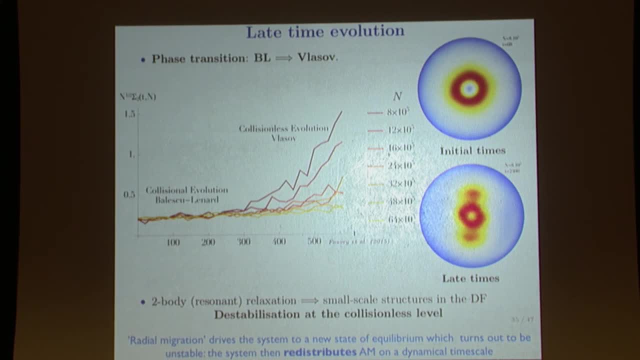 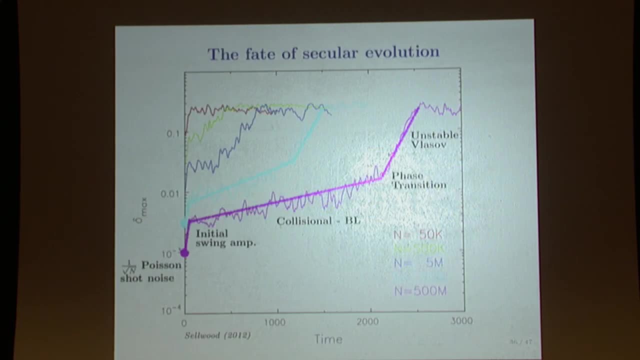 unstable, and so it can rearrange or redistribute its angular momentum much more effectively thanks to the fact that it's built this fridge. okay, so this is was also noticed by Selwood. this is the collisional regime, and then you have a phase transition and unstable Vlasov stage. since I have a bit more time, so 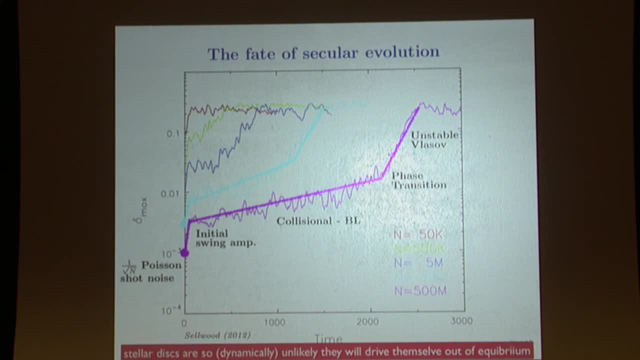 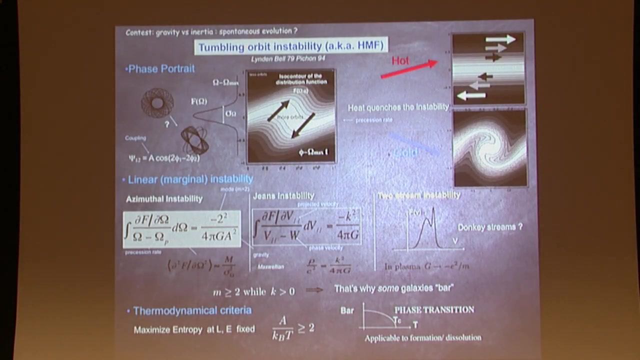 this course. this like so much the state in which they were formed that they drive themselves slowly into a new state where they can just redistribute violently their angular momentum through an instability. which is quite interesting because in the 70s Lyndon Bell wrote a paper on the so-called 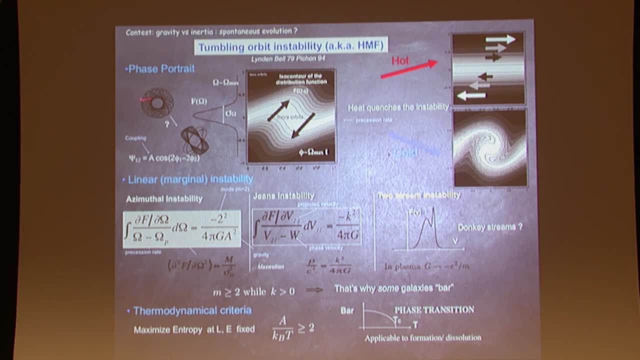 tumbling instability where you ask yourself: how does a such a nice ellipses align each other? if you assume that they all have. they have a certain distribution of angular frequency and you can write down the equivalent of genes and stability for the analog of a gene instability from it, which correspond to an azimuthal. 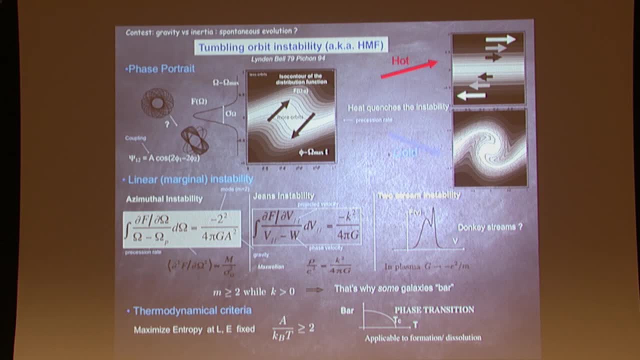 instability of these ellipses aligning each other. and it will happen if the, the temperature, so to speak, and the distribution of angular frequency is sufficiently narrow, so that gravity overtakes inertia, or heat content, if you prefer, and I'll, I'm guessing. I haven't proven this. 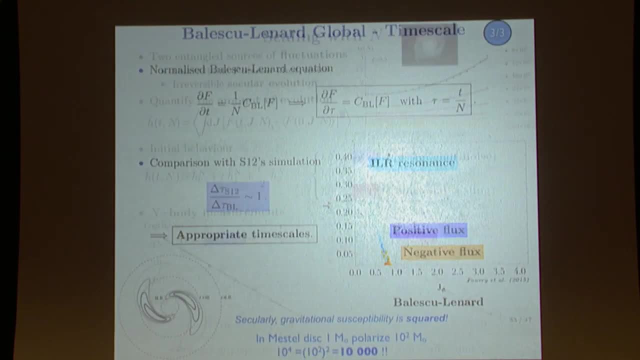 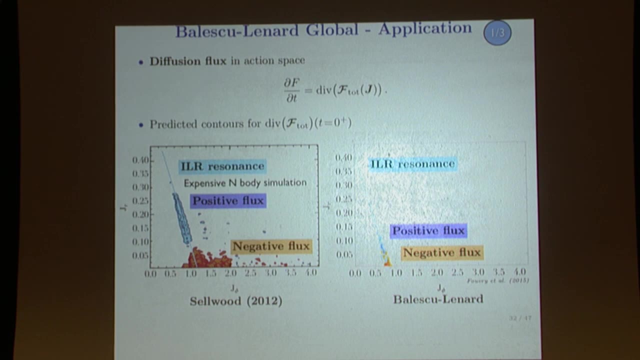 but I'm guessing this is exactly what's happening here, because we are on this ridge which is essentially at a very narrow distribution of angular frequency, So it's almost a test case for a Lyndon Bell scenario of 79 of this tumbling instability. 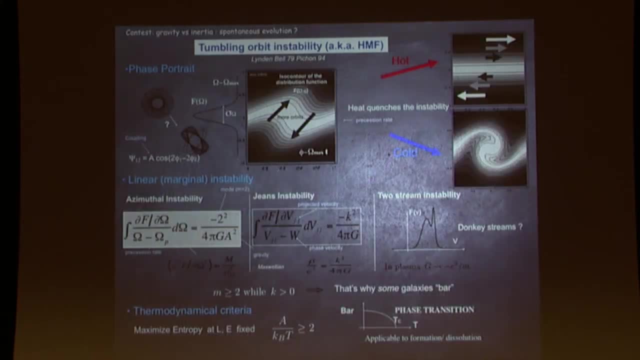 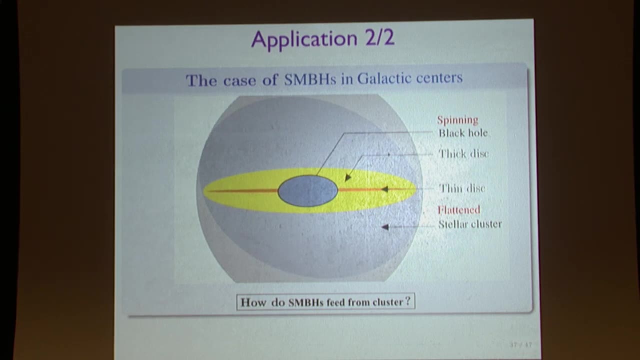 Okay, so I should move on to the galactic center. Okay, Yes, So it's back to your. So we looked at this and we did a multi-species analysis, where you would have a large number of stars and a much smaller number of molecular clouds. 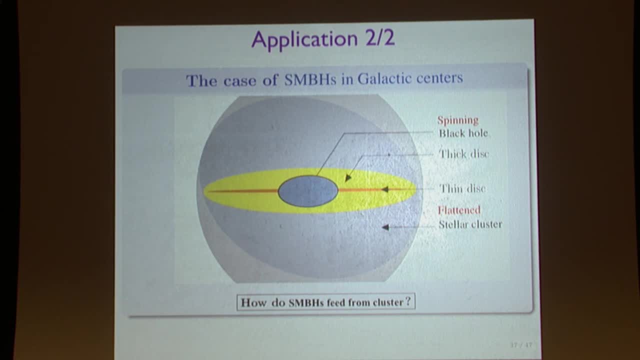 And then the molecular clouds are actually running the show, And I think, at the level of order of magnitude, the number of molecular clouds we had were numerous enough or low enough. What's the reaction of the mass to molecular clouds? What do you do now? 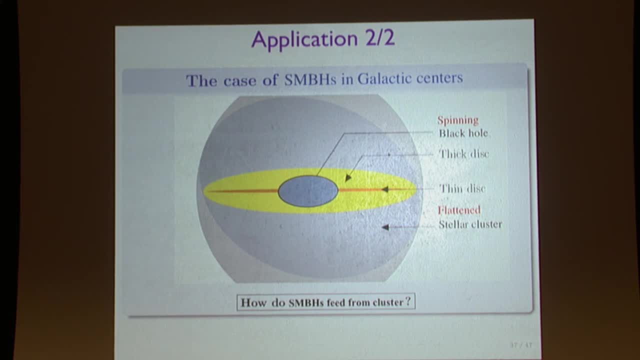 I don't remember. It's not a strong point. Let's put it this way. I'm not trying to convince you. This is relevant to galactic dynamics as such. It's just an illustration of why the formalism works, And we're comparing it to an experiment. 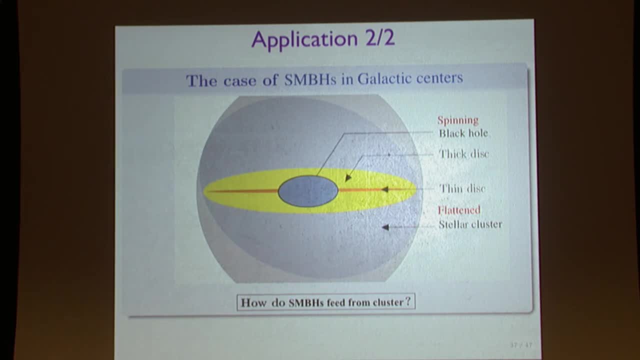 Absolutely. This is an important point for everyone, though. So would you say the following: is true That this process of turning and migrating stars, so a star that's in the currently solar orbit, the solar circle- comes from, for example, four, five, six, four, five? 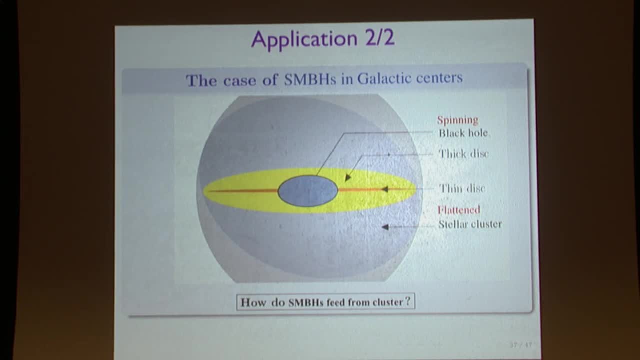 So thank you for asking this. I completely forgot to make this point. Yeah, So what you're seeing, the formation of this ridge- is exactly the process of turning and blurring at the same time. right Blurring would be moving up and turning. 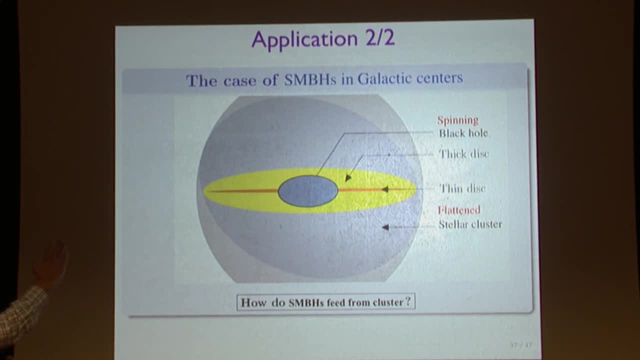 would be moving along the x-axis And we have a. Well, I don't work in this at all, But what people tell me is that the molecular clouds, even though you said so, is low mass, The transient nature of the spiral structure. 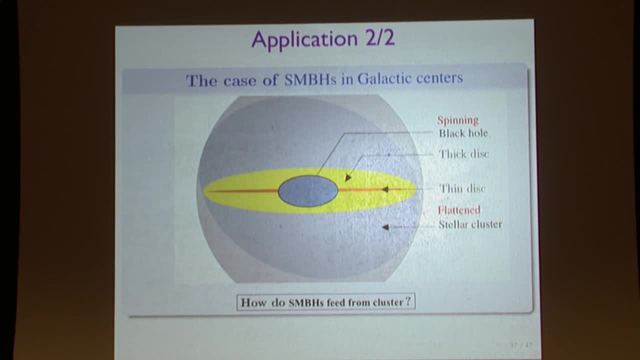 means that you turn and you're anti-turned both times around and you immediately connect them right. So the solar circle is done. Even if you think about the circular orbit, they can have come from a range of initial radius between 5 and 15 new degrees. 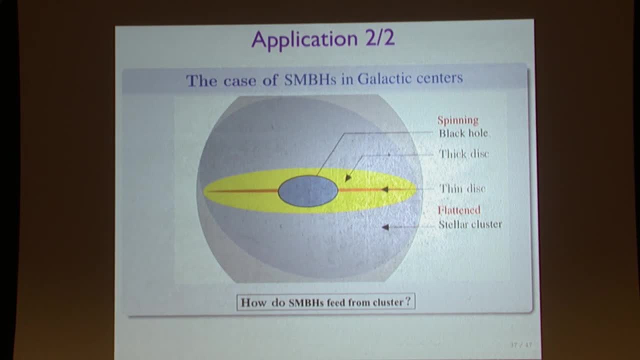 Can I use again my jet lag argument or You can tell me in six hours, Oh, thanks. Another question, same thing. Do you need to? How important is that, especially by government and customer, to bring this data, to get this back? 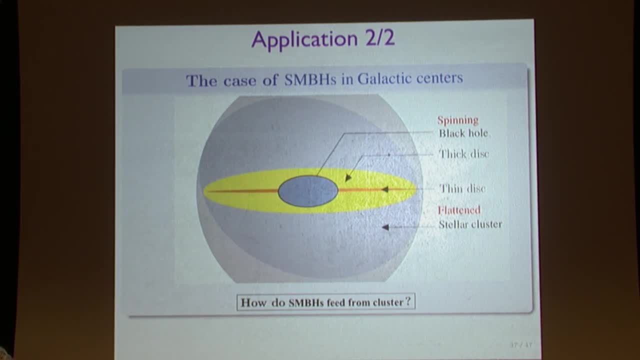 and the government has something to do. and how is it? how important is that compared to whatever you think about what you're saying? That would be impulsive heating, So not described by resonant relaxation, but described by the equivalent of two-body relaxation. 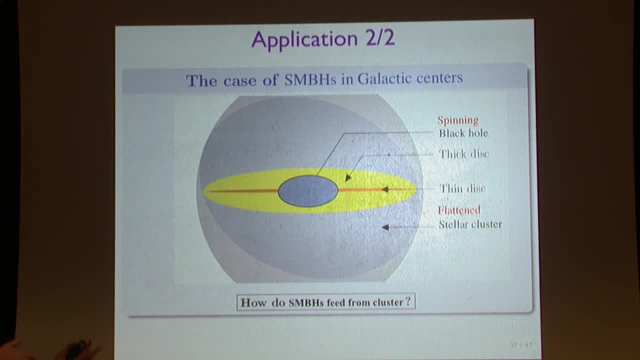 So it would be another source of heating. If you write down the Langevin equation corresponding to Baliscou-Lenard, you would need to add new diffusive term coming from this source of heat. But wouldn't it be enough to camouflage some of the heat? 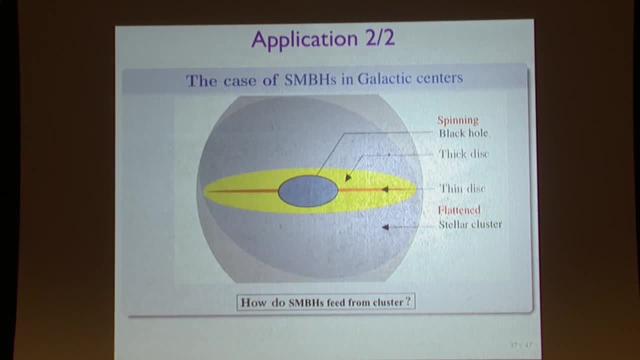 I don't think so. I mean the time of the large micro-thousand in the. There's only a hundred of them in the same. A small fraction of it, Yeah, So it's a micro-thousand in the diffused time. 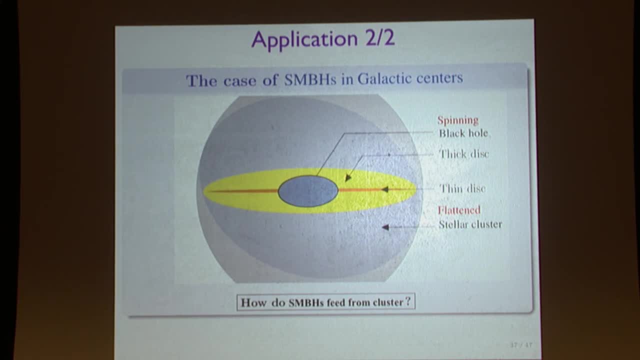 and it's probably 10 to the 3,, 10 to the 4,, 10 to the 3,, 10 to the 5,, 10 to the 6.. OK, So, galactic center. So I'm going to now transpose the general results. 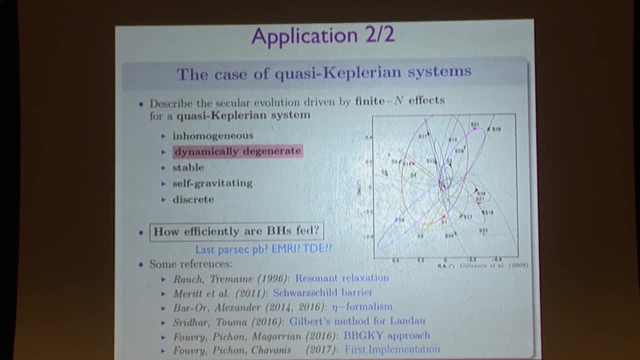 to the case of the galactic center. So the thing which changes is the potential, And the fact that the potential is Keplerian means the frequencies are identical. So in principle, I have a problem in my equations because I have a Dirac with the resonant conditions. 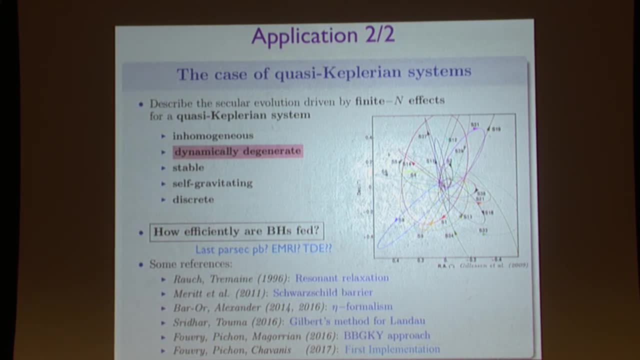 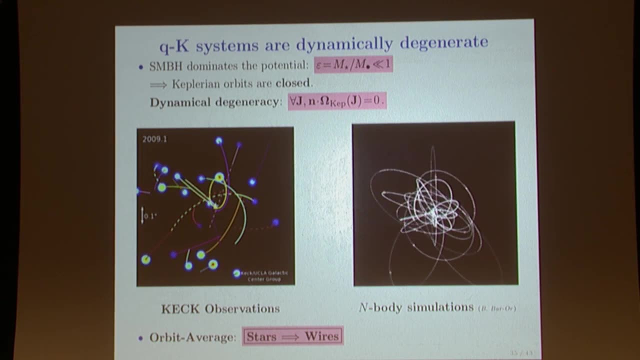 I'm going to have a Dirac with 0 inside. So the way out is to well you know about galactic centers. The way out is to basically do an orbit average before you derive the equation, or as you derive the equation. 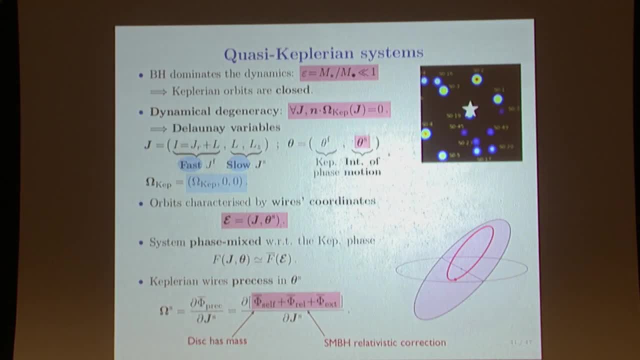 And then you end up with exactly the same equation as before, except that the distribution function you have to consider is the average over the fast angle of the initial distribution function. So you use the relevant angle action variables for the Kepler problem, which are the linear variables. 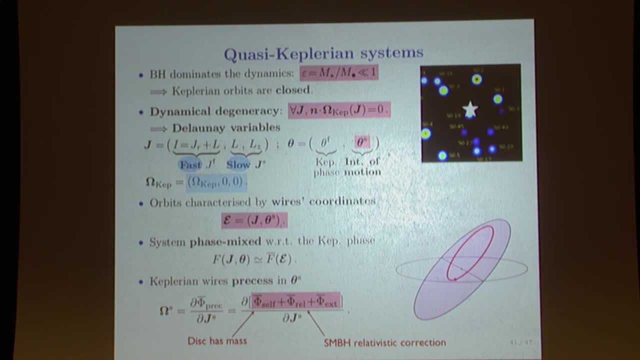 So each orbit is characterized by both by its action and by its slow angle, corresponding to the orientation of the ellipse, And you have a source of precession corresponding to the coupling between the orbits, which is driven both by the self-gravity potential of the fact. 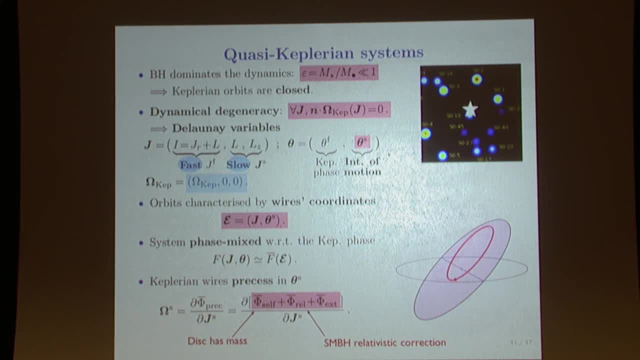 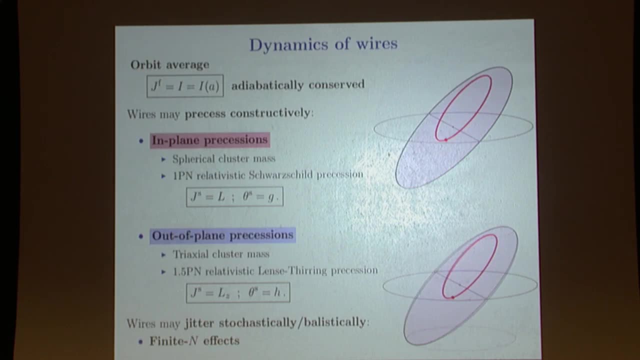 that there is some mass in the distribution of orbits and terms corresponding either to the external cluster or to the relativistic corrections. So these are my new frequencies And I can have two situations: either I have in-plane precession or out-of-plane precession. 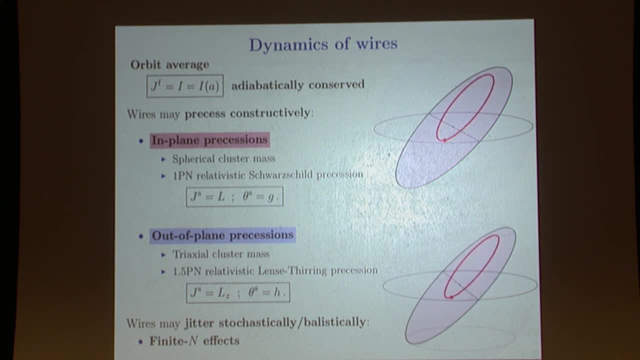 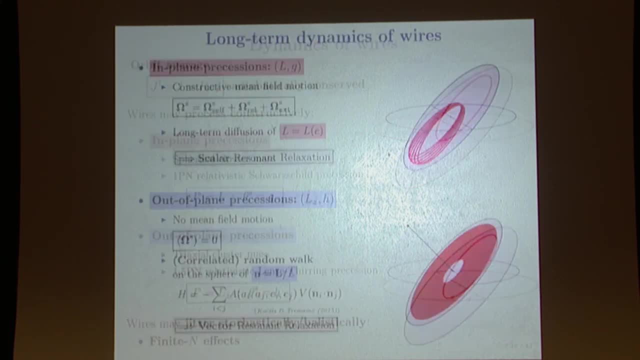 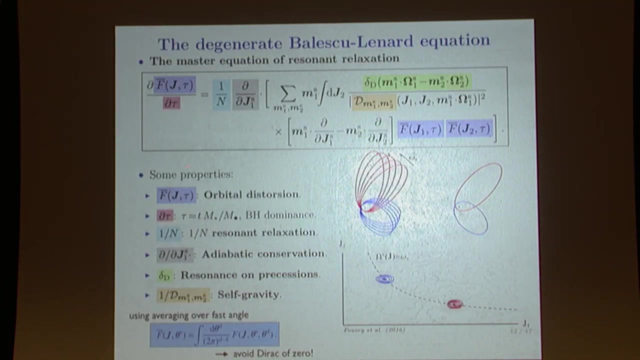 depending on the nature of the environment. Is my black hole rotating or not? Is my external cluster spherical or not? And I guess, well, you know this better than me, so let me just skip this. So this is the equation of exactly the same equation. 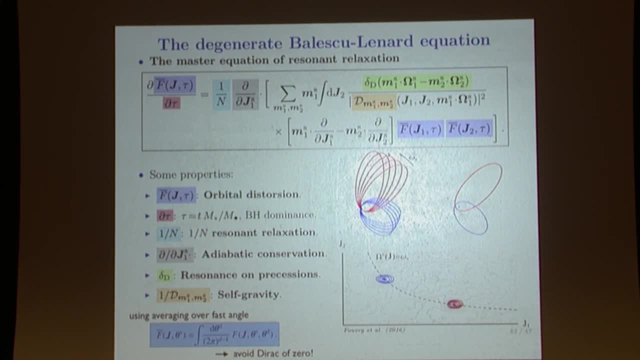 as previously, except this time I have bars, which means that I have average average over the first angle, And so the question here is: is a fluctuation in the number of wires at this frequency allowed to talk to another fluctuation at the same resonant frequency? 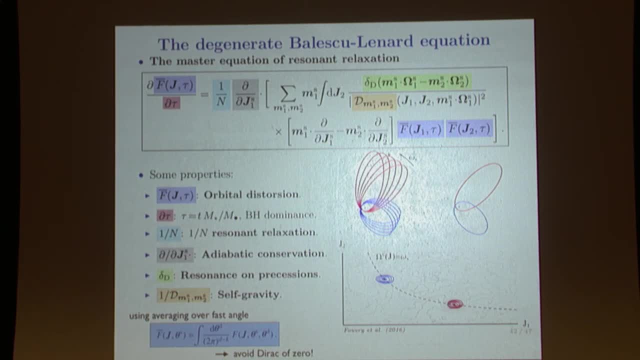 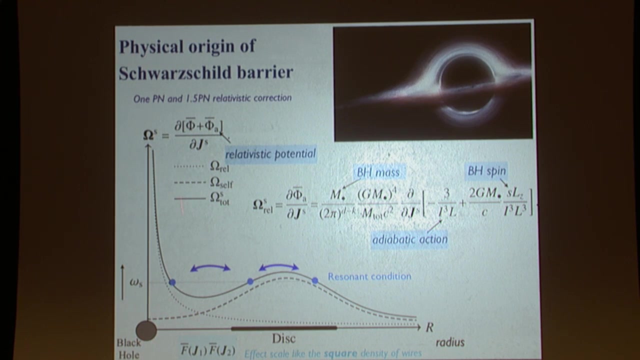 so that the two set of ellipses can talk each other through the variation of the potential due to the relativistic effect of the black hole and the mass in the disk. So this is nice because it explains quite naturally the emergence of a Schwarzschild barrier. 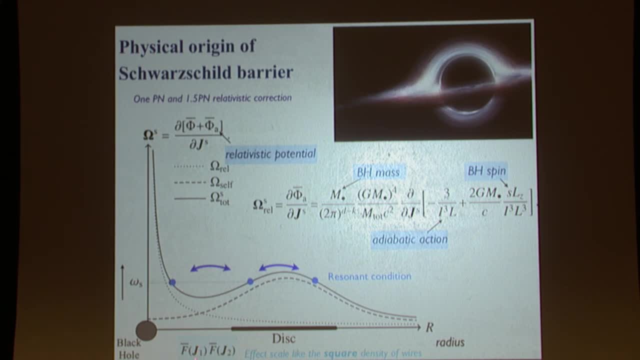 because for the process to work we need to have a coincidence of orbits which have the same frequency. So if I am far enough from the black hole so that I have a frequency which is below the local maximum here of the frequency as a function of radius, 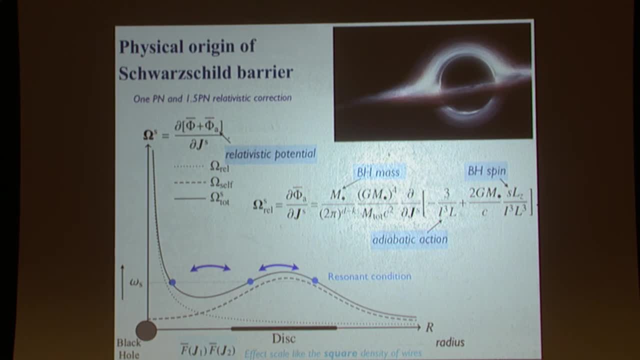 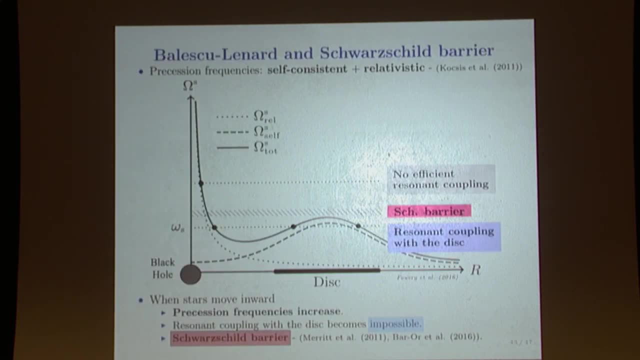 which is dominated by the disk in this region and dominated by the black hole here. then I can find pairs of wires which can talk to each other, but as I reach an inner region such that I can't find any more pairs of orbits to talk to each other, 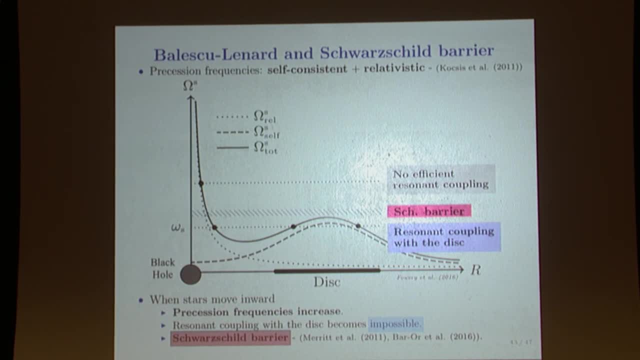 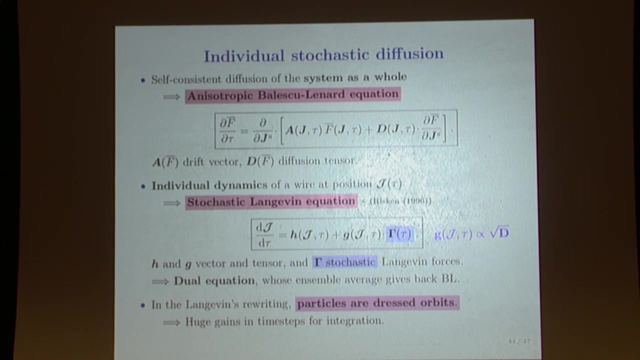 then the diffusion process stops and the diffusion coefficient become zero, and so I recover, very naturally, the Schwarzschild barrier with the Balest-Coulénard in the context of galactic centers, Because they don't have anybody else to talk to, They need to talk to someone else. 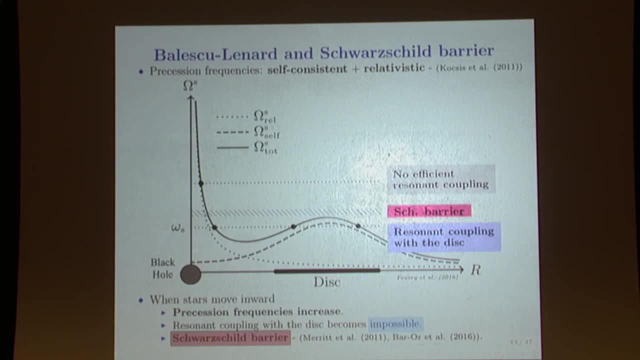 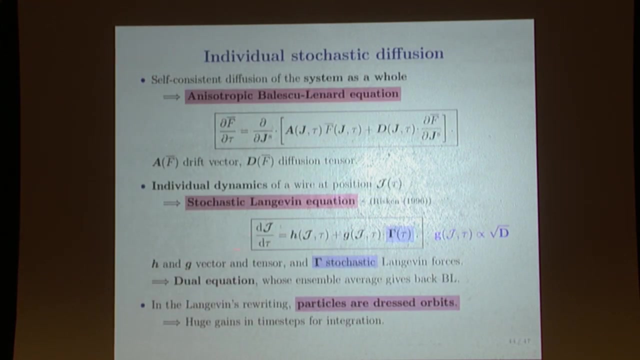 And, Yes, One minute, So I can write the corresponding Langevin equation, which is a classical trick of transforming a Fokker-Planck-like equation into the equation for the underlying particles, if you want, which is driven by a stochastic force. 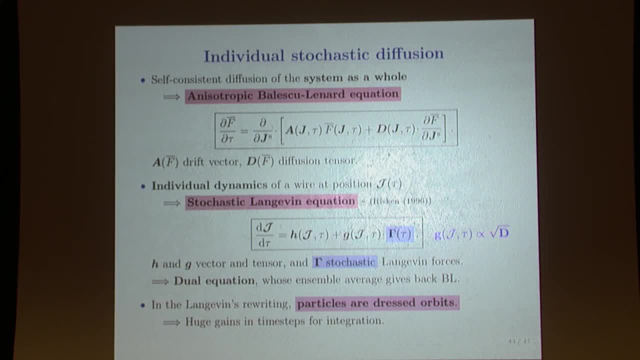 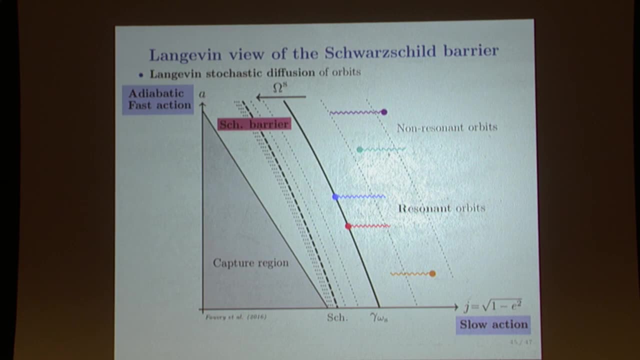 and which involves the square root of the diffusion coefficient as a driving pre-factor for the stochastic force. And so, in this formulation, then, depending on whether my two set of wires are resonating or not, they will be able to talk to each other or not. 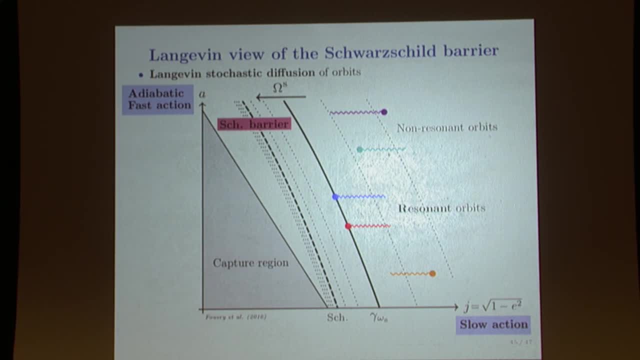 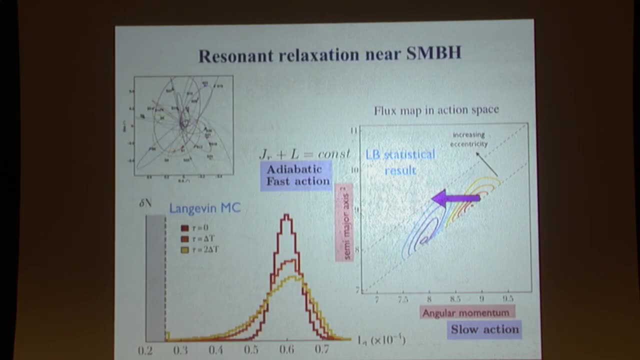 And so you see here the Schwarzschild barrier here corresponding to the fact that the frequency is becoming too high, And two more slides. So this is an implementation once again of the full formalism in the context of the Kepler problem. So here I'm looking at again. 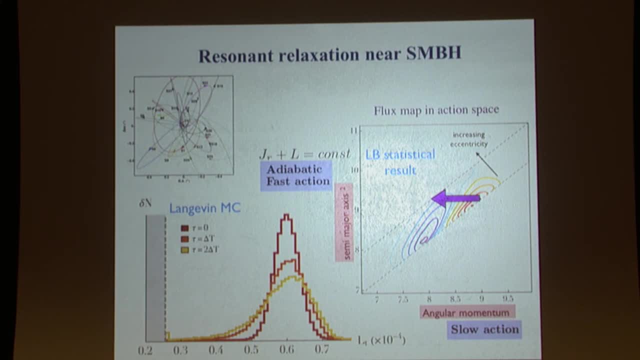 a map representing the depletion and excess of wires induced by the diffusion process, as computed by computing the diffusion coefficient of the Balestrelian equation. So you find the known result that the semi-major axis is adiabatically invariant and you have an increase in eccentricity due to the fact that some of the orbits are going to torque. 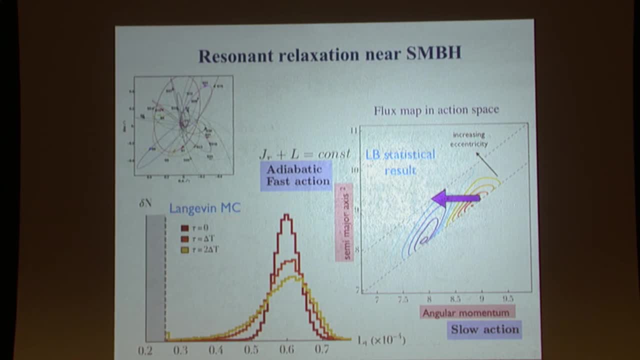 each other. And if I do a Langevin implementation of this, then I will find the same process of the fact that my initial distribution of stars will broaden itself and the diffusion process will stop at the Schwarzschild barrier imposed by the presence of the black hole. 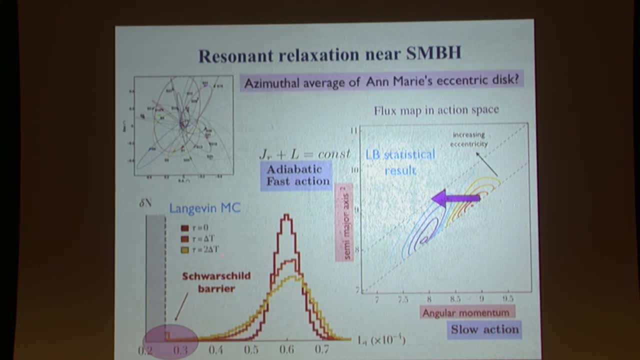 And so I believe- but this is last night's lack of sleep because of jet lag- that this is quite relevant to the talk of Anne-Marie yesterday, where she was looking at this eccentric disc and finding that the self-interaction of the Ys would allow them to pump up eccentricity. 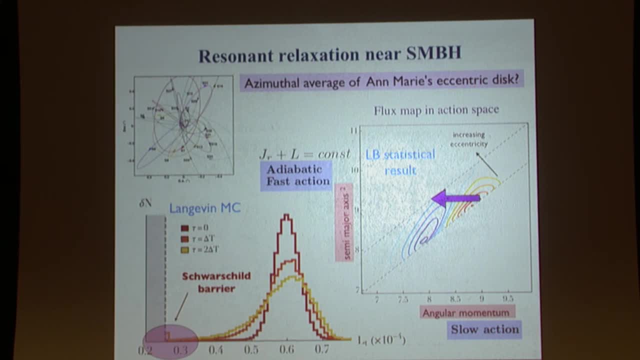 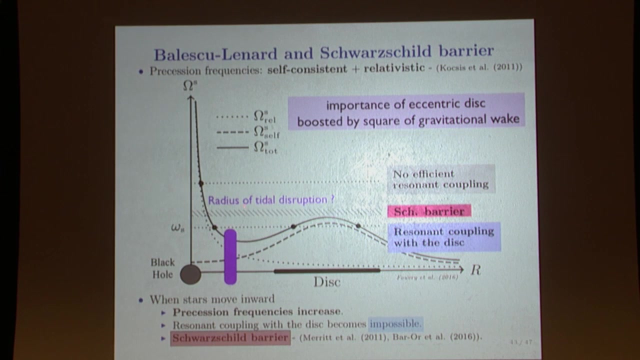 and trigger tidal disruption. What's the last acronym? It's an acronym with three letters: tidal event. And so what's important here is that in the Baliscouline formalism you have this gravitational amplification coming from the gravitational wake of the orbit. So if your disc is sufficiently, 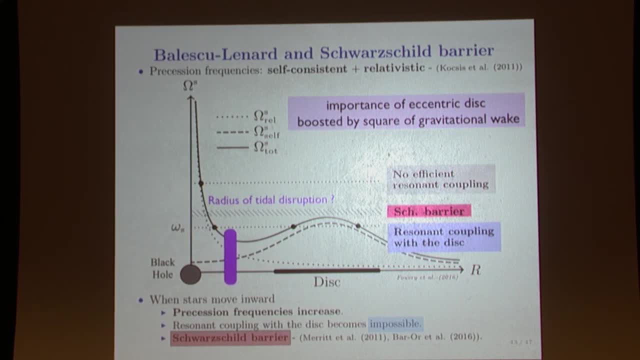 massive and she had a disc which was not, which had a mass which was not negligible compared to the disc. The process of eccentricity pumping will be strongly boosted by the self-interaction of the orbits. So I guess this is something to be discussed.